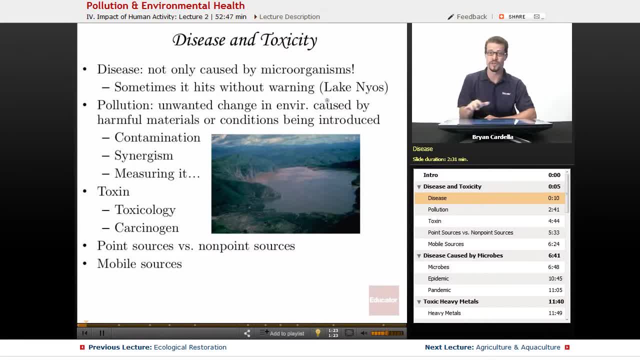 and is completely out of control. So it's not just one cause, one effect. It's completely non-discriminatory in terms of who it affects, And an example of that is a tragedy that happened in Lake Nyos in Africa. The tragedy at Lake Nyos was such that, because of natural occurrences in the earth, 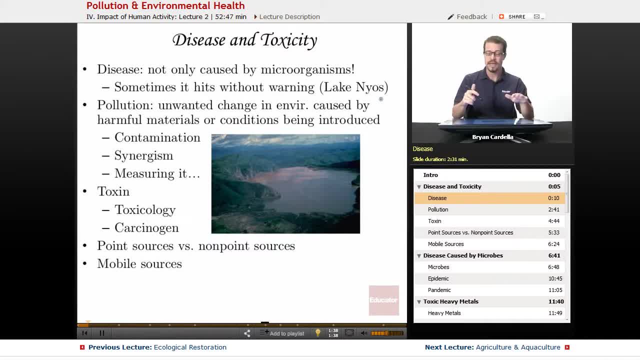 a lot of CO2 built up at the bottom of a lake And it happened to sit low in the water. But because of a disturbance, some geologic activity, maybe earthquakes and such that gas was pushed upward got out of the water. 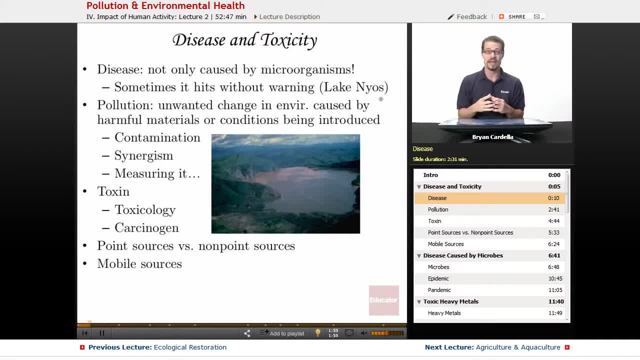 down the mountainside into the neighboring town And, because that particular gas happens to be heavier than the rest of the air combined, it was just sitting in the town and it killed over 1,800 people due to asphyxiation, And that's a tragedy, of course. That's just. it didn't discriminate, It just killed a lot of people. 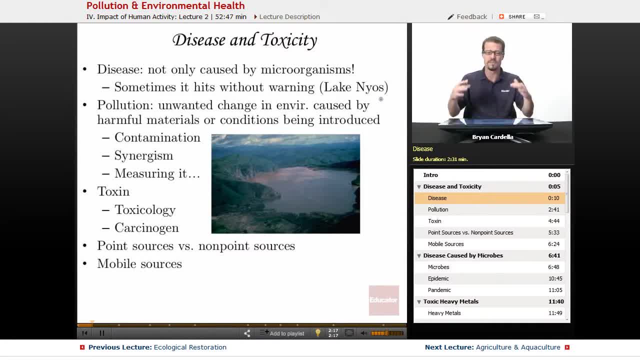 And so there's been attempts to solve that problem. What if this buildup happens again and several decades later the town is harmed once again? So there have been pipes that have gradually been installed in the lake to try to draw out the CO2 and release it into an area where it's not going to be as harmful. 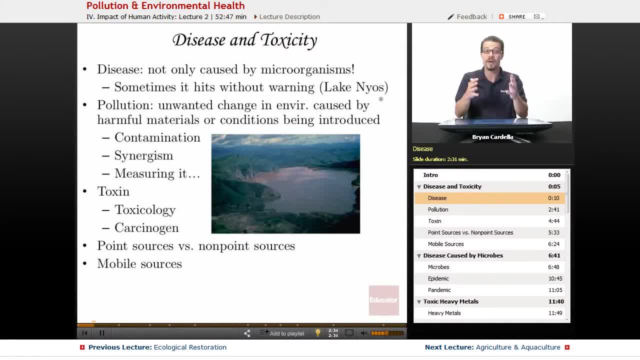 The amount of work that's been done so far hasn't done that much to solve the problem completely. So it's a work in progress and hopefully that tragedy won't happen again. Pollution is an unwanted change in the environment caused by harmful materials or conditions being introduced. 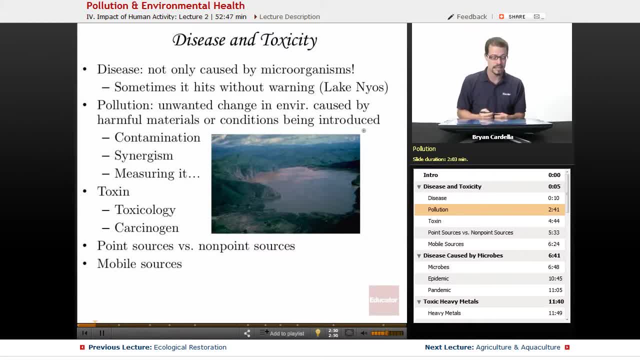 And oftentimes we're talking about a man-made cause or human-made cause. Pollution is an unwanted change in the environment caused by harmful materials or conditions being introduced, And oftentimes we're talking about a man-made cause or human-made cause. Contamination is an unwanted change in the environment caused by harmful materials or conditions being introduced. 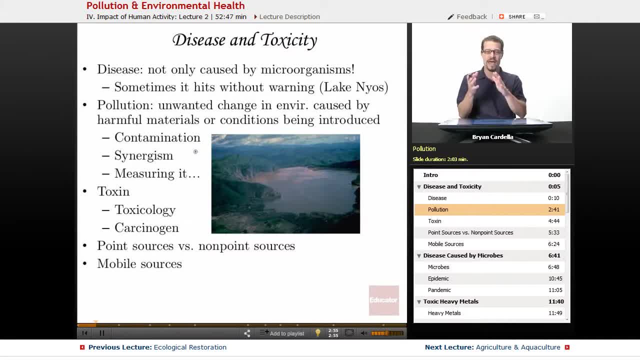 And oftentimes we're talking about a man-made cause or human-made cause. Pollution is an unwanted change in the environment caused by harmful materials or conditions being introduced, And oftentimes we're talking about a man-made cause or human-made cause, But with contamination we're talking about that specific pollutant or contaminant being in a particular solution or air supply. 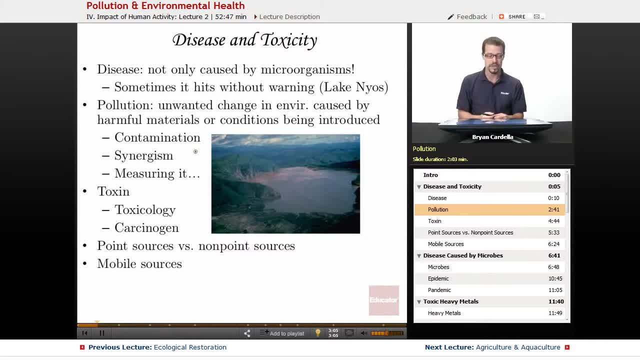 If we're talking about: oh, our water is contaminated, we're saying it is polluted with a particular substance. A synergism is the case where you have multiple pollutants or contaminants together whose effect is greater than the actual sum of their parts. For instance, you could have 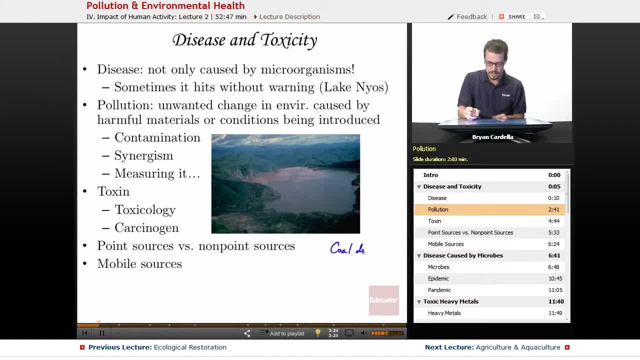 I don't know, I don't know, I don't know. coal dust and this particular compound individually cause problems with the lungs, but when these two combine, when you get so2 combining with coal dust, it actually can end up deeper in the lungs. the dust allows it to travel. 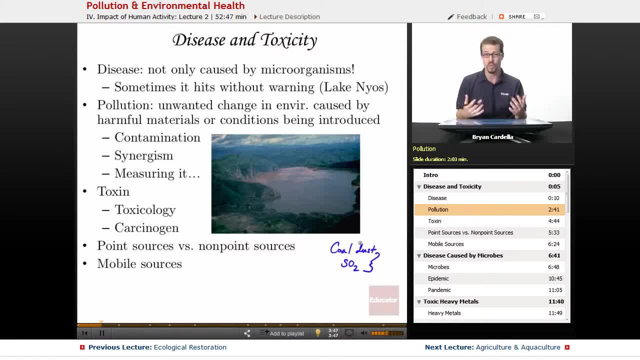 deeper and the combined effect can be much worse than those two independently. so synergism can happen when you get different toxins or pollutants combining, measuring them: there's particular ways to measure them. you could say parts per million, that's in ppms, meaning if we had a 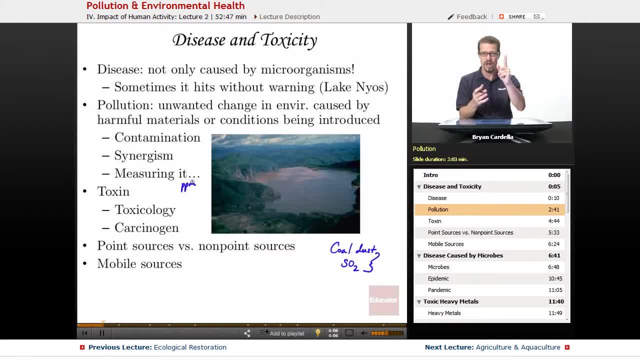 million molecules and there's one ppm. that means one of the molecules out of a million. is that particular compound? or it could be even ppb. uh, parts per billion. and, by the way, parts per million is actually like saying one milligram per kilogram of material. it's, it's the mathematical equivalent. 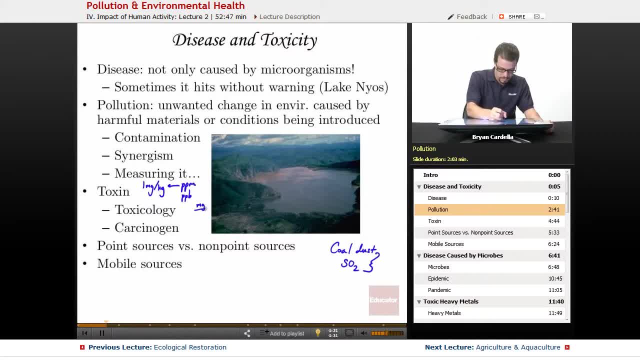 uh, you could also do it with hey milligrams per liter. maybe we're talking about a certain compound dissolved in water. whatever it might be, there's various ways for measuring how much of a pollutant is found in a material. a toxin? a toxin is really um any harmful substance that ends up in the 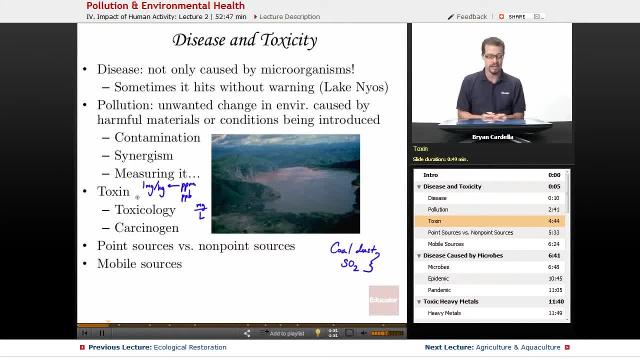 in the environment that can harm a human being. there's some other ways to measure it: uh, human, animal, plant, really any organism. So toxicology is the study of those toxins in the environment and the effects they have on animals, plants, etc. A carcinogen is a toxin that. 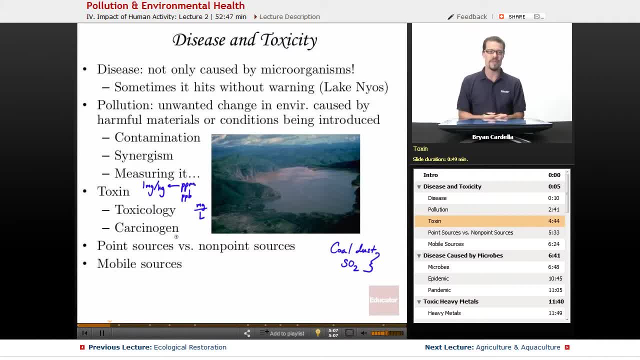 specifically, is known to cause cancer. So something about that particular toxin has the potential to change genes that actually regulate the cell cycle in organisms and lead to having tumors develop- benign or malignant tumors, Malignant being the more harmful, of course, Carcinogens. I've read. 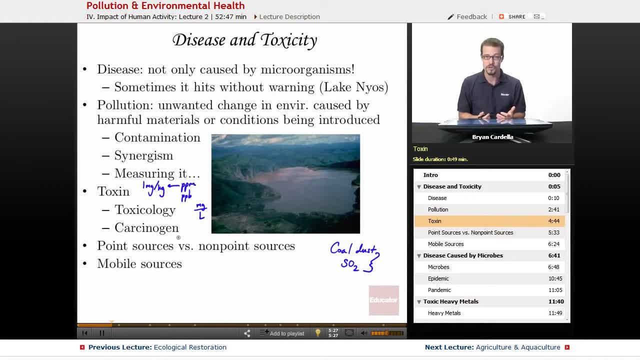 that in cigarette smoke there's actually over 100 separate carcinogens, which is a scary concept. When it comes to a release of a toxin in the environment, you can have point sources, meaning it's a specific source that has one particular point. So a point source could be. 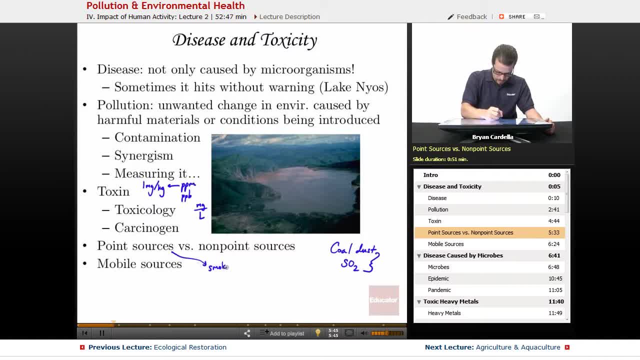 a smokestack. From a smokestack at a factory, there could be a lot of different toxins being released. Maybe it's an oil spill. That's a specific area, a point that originated Non-point sources, also called area sources. 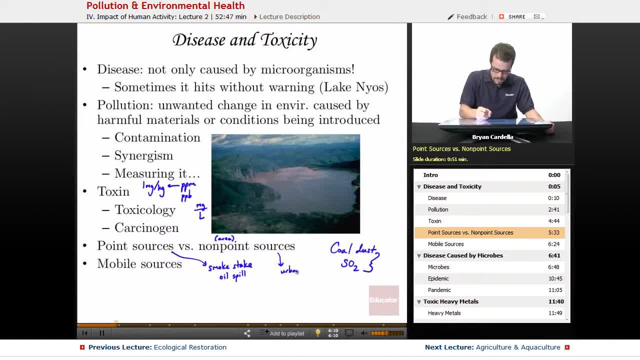 An example of this is urban runoff. So, yeah, it does have a particular origin, but it tends to be more widespread with how it's diffused. So it's a specific source. So it's a specific source. So it's a little bit more widespread than something known as a point source, Mobile sources- they move. 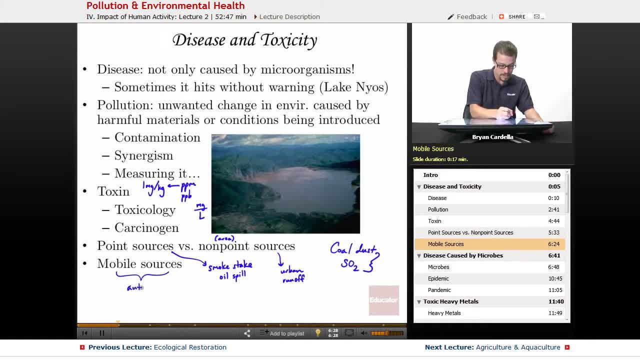 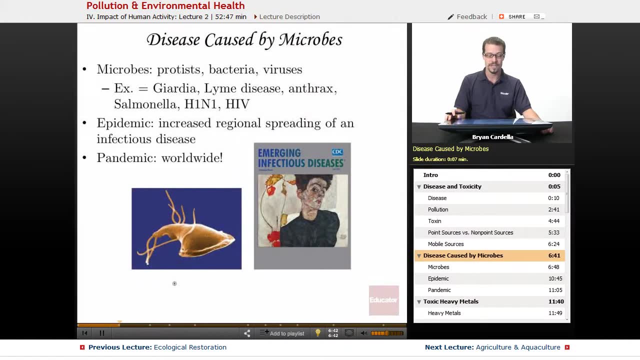 A great example of a mobile source is auto or car exhaust. Cars move around. That's what they're designed to do, So that's a mobile source in terms of something being released in the air that could be harmful, All right, And you know, there's also disease, of course, caused by microbes, not just pollutants. 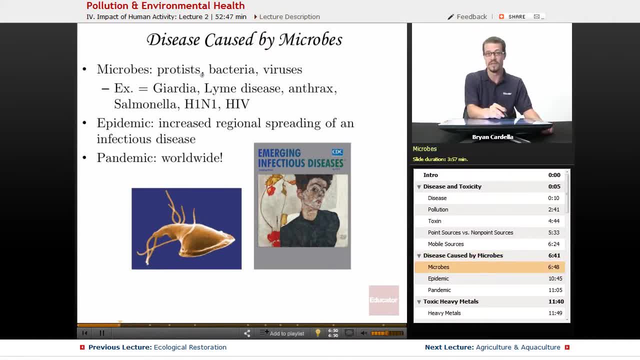 but toxins. Microbes include protists. These are technically eukaryotic cells like ours, but oftentimes they're just one cell on its own. They can be multicellular, but generally the protists that cause problems in humans are microscopic, made of just several cells or maybe a few hundred. 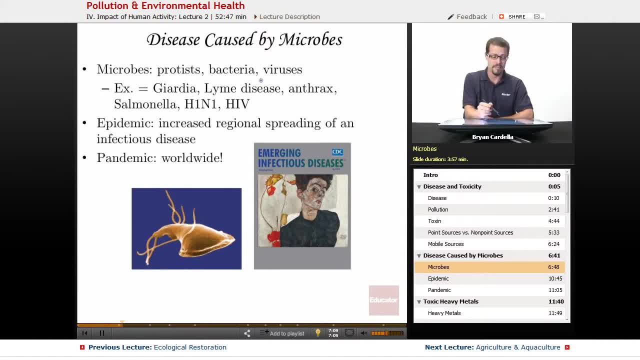 at the most: Bacteria. Bacteria, single-celled beings that are prokaryotic, and bacterial infections plague millions of humans every day. Viruses, Of course. viruses. those are the tiniest of those three. They're technically not even made. 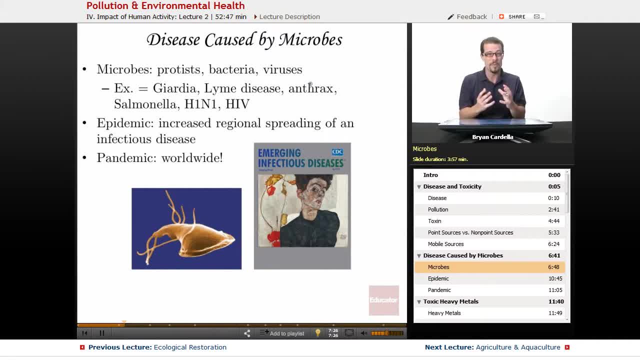 of cells. They're kind of like little organic robots, just DNA and RNA or RNA wrapped up in a protein shell. Examples a protist infection: Giardia. That's depicted right here. Giardia causes intestinal problems and if not treated it can kill a person. Lyme disease- Lyme disease. 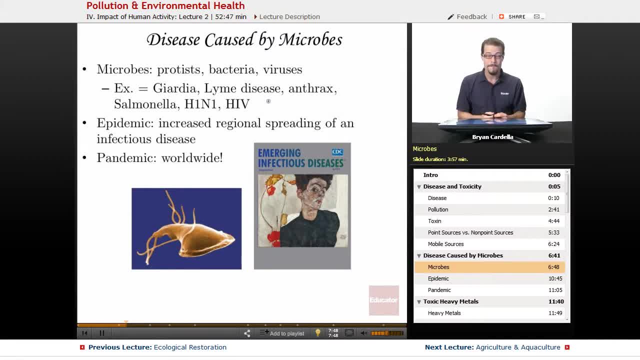 is caused by a bacteria that's usually communicated or transferred to a person by ticks. So if you're hiking you have certain parts of your skin exposed, it's possible for a tick- a deer tick- perhaps- to land on your skin, bite you, and if it has that bacteria inside of it, it can transmit that into your bloodstream. 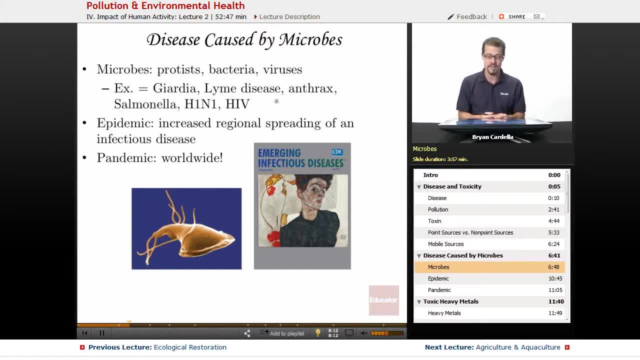 It can cause permanent nerve and muscle damage and, if not treated, it can actually kill a person. Anthrax is also bacterial. Let me actually color code these bacteria: bacteria bacteria. Yeah, actually anthrax is Bacillus anthracis. That's the common form of bacteria that causes anthrax. Um, a lot of times it comes out of your blood as a suspected condition and instead does cause sudden true malformations. Um, a lot of times it comes out of your blood as a suspected condition and instead does cause sudden true malformations. Um, a lot of times it comes out of your blood as a suspected condition and instead does cause sudden true malformations. 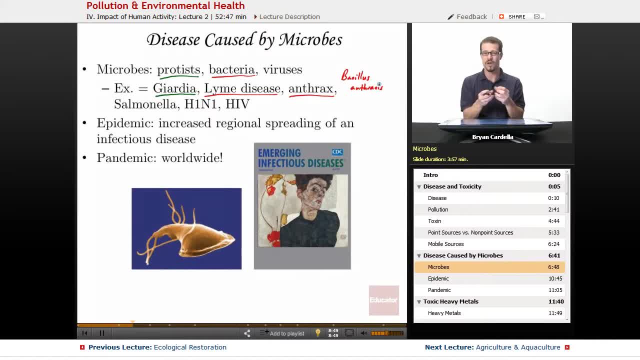 times it comes in like an endospore form, a dehydrated, almost like white powder looking substance, and this is something you hear about in the news. if somebody wants to engage in terrorist, terrorist activity and send an envelope to somebody to open, when they open the envelope, if they inhale those spores, 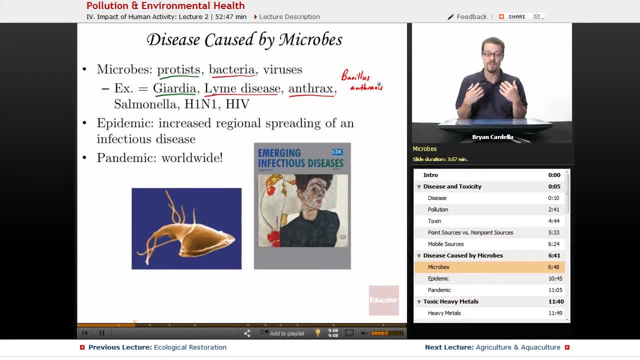 those endospores. as soon as they come in contact with mucous membranes, you can get the bacterial infection and, if untreated, it can kill a person fairly quickly. salmonella also bacterial. this is a genus of bacteria. it's usually associated with poultry eating raw chicken or raw eggs. that's not the only place it's found. that's just where the 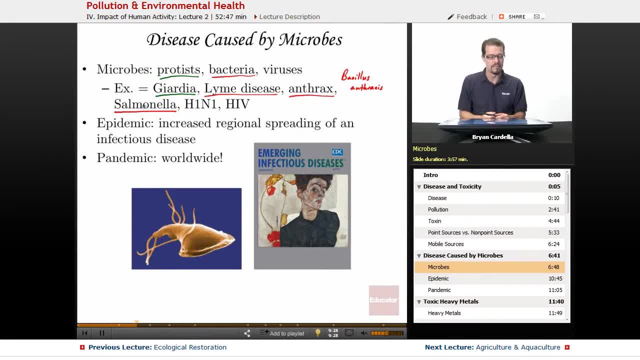 average person is most likely to be introduced to salmonella. there's been salmonella outbreaks where it's been found extensively on certain crops and actually ends up on spinach or in other things that have gone to market and there'll be a recall if it's discovered with viruses. 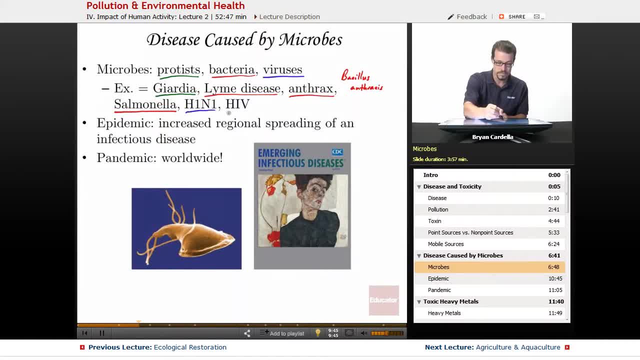 let's use blue h1n1, of course. there was a famous worldwide outbreak a few years ago with h1n1, also known as swine flu. the thing with h1n1 is the form that ended up in humans and infecting human. human human ended up actually having markers for two forms of swine flu: one. 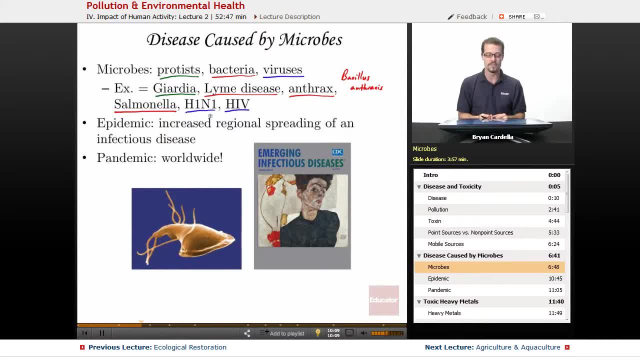 form of human flu and an avian flu in it. so really, with increased exposure to livestock close quarters, these kind of outbreaks could be happening more and more over time if we don't figure out a way to reduce that exposure. HIV, of course, is also viral. human immunodeficiency virus can lead to AIDS, and it's something that 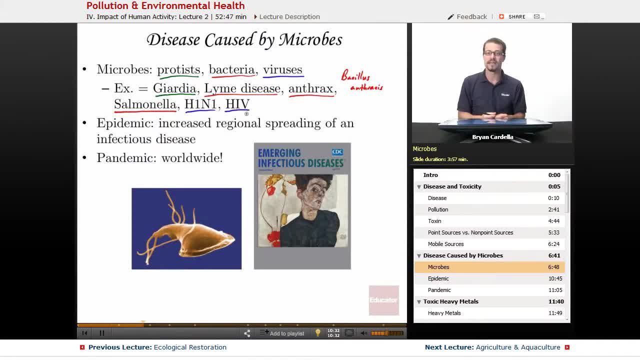 has a virus that actually attacks t-cells, a kind of white blood cell in the human body. there's also simian immunodeficiency virus, but this is the human form anyways. an epidemic is an increased regional spreading of an infectious disease. so there are infectious disease diseases that are just out there and we 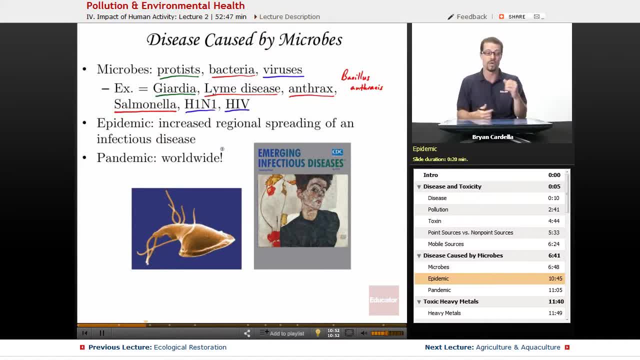 have sort of expected exposures or or an expected kind of rate of contagiousness that that you know we've come to live with. but an epidemic is beyond that, where it's an increased spreading. that is somewhat of a surprise and actually can lead to a pandemic pan, meaning worldwide. 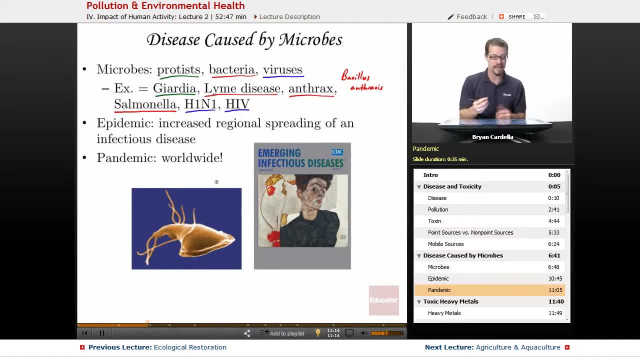 that pandemic. an example of that in 2009 with the H1N1, the swine flu, SARS, bubonic plague- you know the Black Death in Europe. so with a worldwide outbreak it becomes a pandemic. so here's actually the cover of a recent issue of the 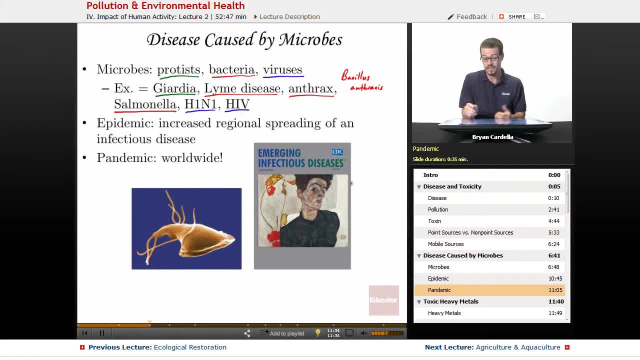 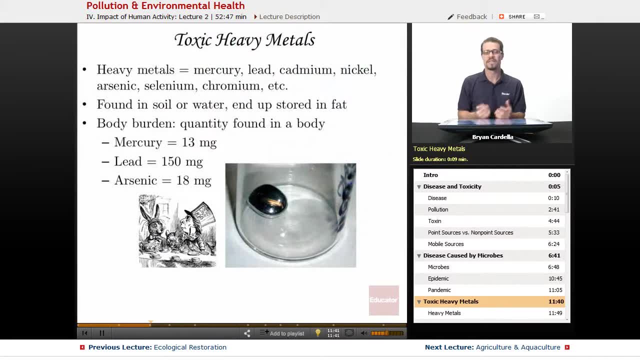 Center for Disease Control emerging emerging infectious diseases. so this is something that scientists and doctors should probably keep up on. toxic heavy metals. these are definitely pollutants that can lead to environmental problems and disease in humans. so with heavy metals, these are the major ones: mercury, lead, cadmium, nickel, arsenic, selenium, chromium and 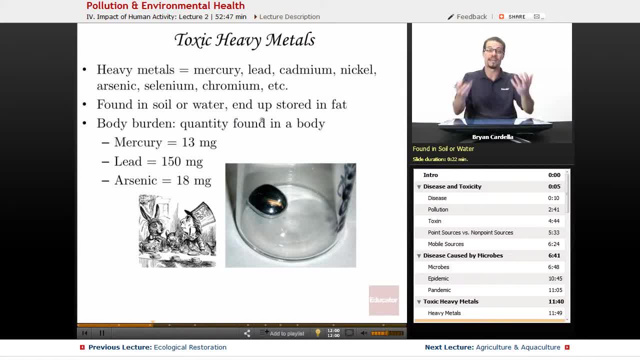 there's others. these are found in soil or water, and if they end up in human bodies, they typically end up being stored, in fact, and fat is found all throughout the body. a lot of it is going to be between the skin and the muscles, that, that subcutaneous layer also known as the hypodermis, but of course, fat is found all. 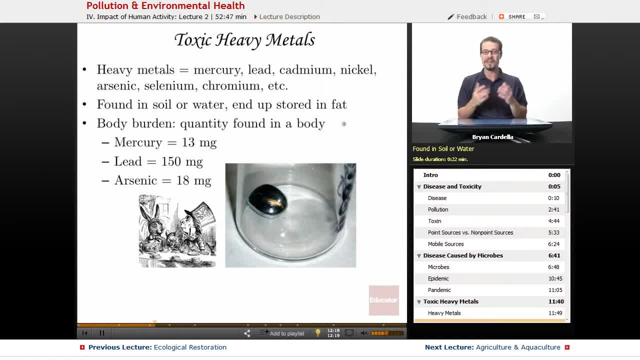 throughout the body. It's very common for these to be in human bodies, in your body and my body. So there's this concept known as the body burden. I have a body burden, you have a body burden. So this is the quantity found in a typical body With mercury, the average human has about 13. 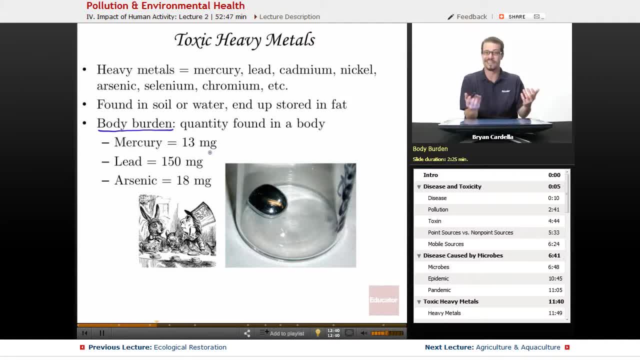 milligrams. This is not enough to kill you. This is actually just an expected amount. Mercury is in the water, It's in the ocean, ends up in fish. Even if you haven't eaten fish before, it's probably in your body Lead. it's expected that the average person is going to have about 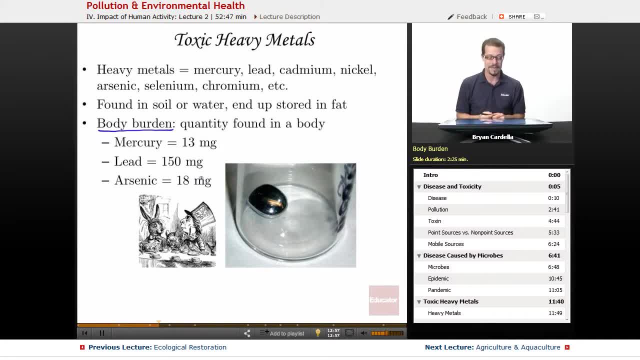 150 milligrams of lead in their body. The amazing thing is that lead. there's actually been many attempts in recent decades to reduce the amount of lead used in products that we use, But lead in the history of human civilization is so widespread in terms of its use that it's just 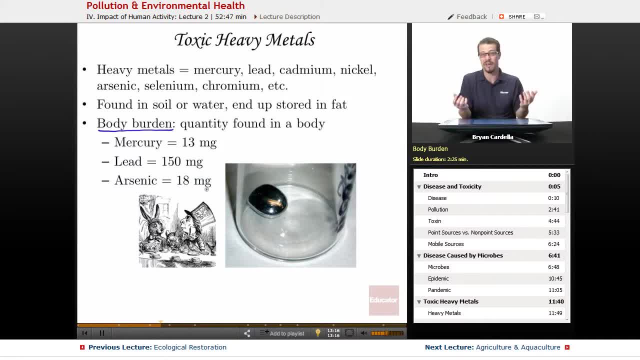 it's in the average human And arsenic 18 milligrams found in the average human adult. So if you're freaking out about this, don't worry, These quantities are not enough to cause disease. You eventually can get to a point where you've exceeded the threshold, meaning, and I'll talk. 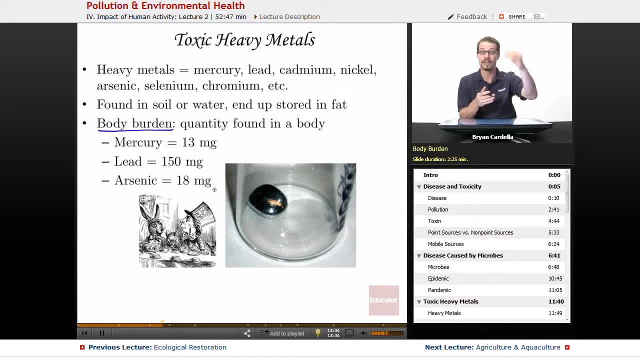 about that more later in the lesson. meaning: from that point on, any additional little bit is going to cause disease. So if you're freaking out about this, don't worry, These quantities are not enough to cause disease. You eventually can get to a point where you've exceeded the threshold. meaning: 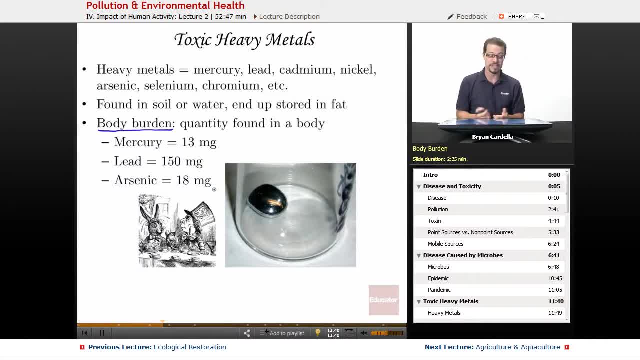 to cause some kind of negative effect, For instance with mercury. though the average person has mercury in their body. if you were to take this liquid metal mercury right here and roll around in your hand and play with it a bunch, well, you'd end up getting a lot more seeping. 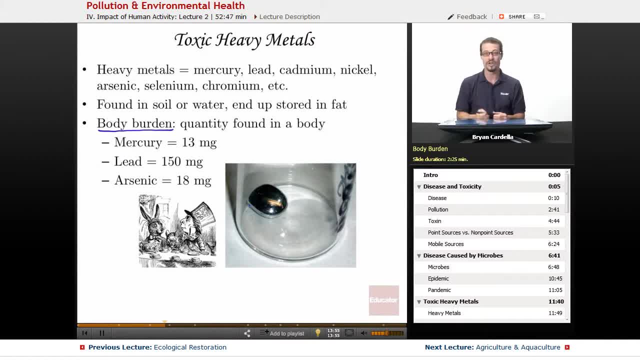 into your bloodstream and into your body And that kind of exposure could negatively affect your brain and potentially make you go crazy. And actually that stereotype or that classic character known as the Mad Hatter from Lewis Carroll's Through the Looking Glasses or Alice in Wonderland- he has come from some anecdotes in history about mad hatters. 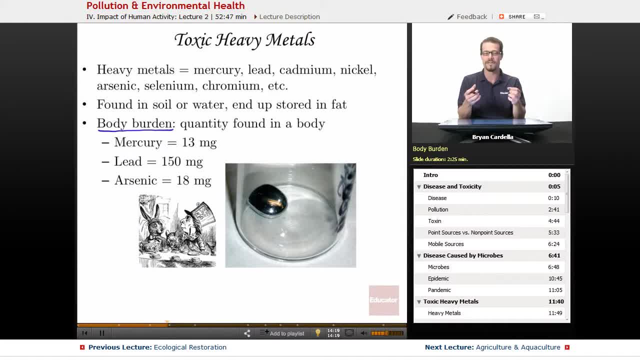 that there actually was a lot of mercury being used to stiffen felt hats in the 1700s, 1800s And at the time they didn't realize that was a bad thing, that it was toxic to these people over time. So these people making the hats, their exposure to mercury was way more than 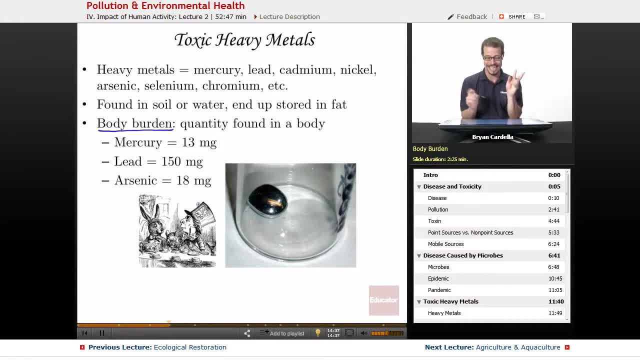 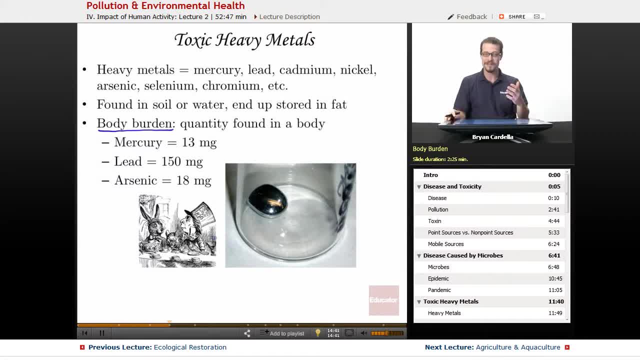 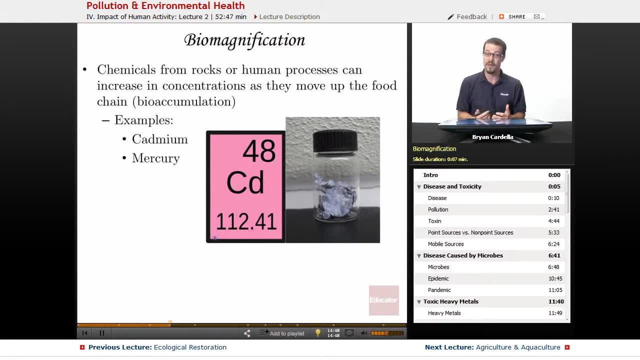 so that's how you get the Mad Hatter. It's kind of funny when you find out fiction has its roots in reality- Biomagnification. So biomagnification is a phenomenon that's been studied a lot over the past couple of decades. Chemicals from rocks or human processes can increase in concentrations. 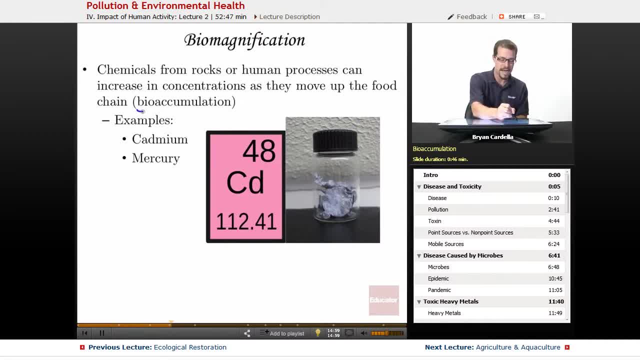 as they move up the food chain. This is also known as bioaccumulation, depending on the textbook you look in, But either way, biomagnification, bioaccumulation. I don't know if you've heard of it, But either way, biomagnification, bioaccumulation- I don't know if you've heard of it. 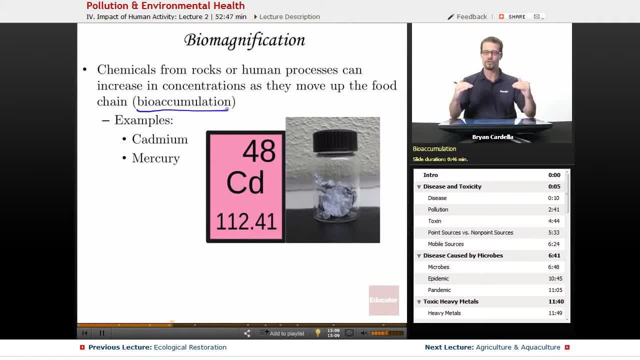 But either way, biomagnification, bioaccumulation- I don't know if you've heard of it- This has to do with just moving up trophic levels. When you start with introduction of some kind of chemical, some kind of toxin, into the water supply, that's going to inevitably end up in plant life, right? 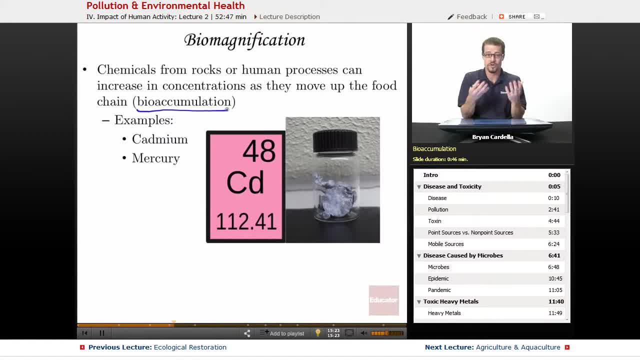 Plants. we all rely on plants. They are the autotrophs, They are the producers. And as something eats the plants, some kind of herbivore eats the plants, some omnivore or carnivore eats them, and so on and so forth, it increases in concentration as it moves up through. 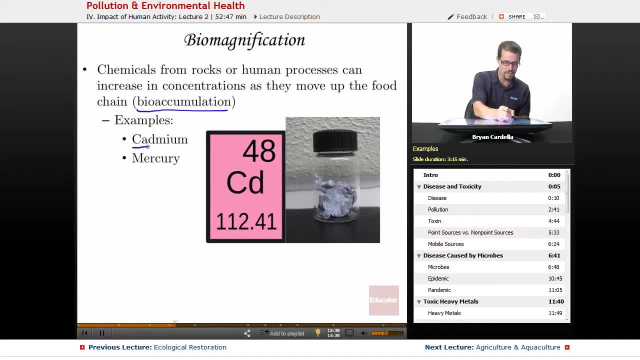 plant life, And so you know it's kind of like you know it's kind of like you know it's kind of. So some examples: Cadmium, If you're wondering what's so bad about cadmium ending up in my body. 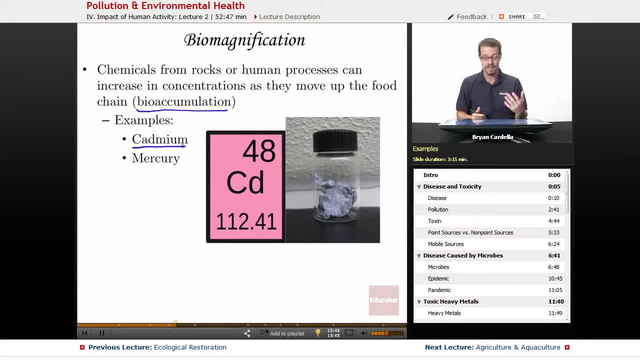 Well, there's already a little bit of cadmium in your body. However, enough of it has been known to cause heart problems. Specifically, the risk of heart disease goes way up. And if you're wondering, well, how do I get introduced to this thing called cadmium that has 48 protons in this atomic weight? 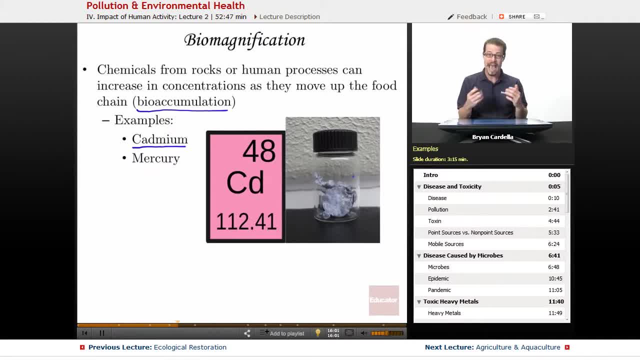 and happens to look like this in that jar. Well, cadmium is found in coal dust or coal ash. So in the United States there's a lot of coal burning And that ash is basically a waste of burning coal to create electricity typically. So usually the coal plants, they'll do something. 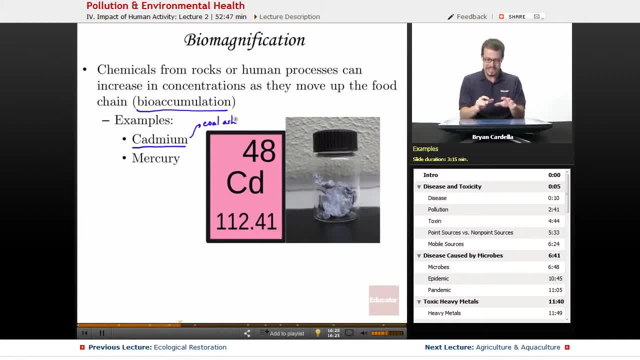 with that ash They'll bury it. They'll bury it very deep in the earth, But it inevitably ends up in the plant life that results in that soil. So in the plants it ends up this cadmium. And then you have, you know you have a lot of coal burning, And so you know you have a lot of coal burning. 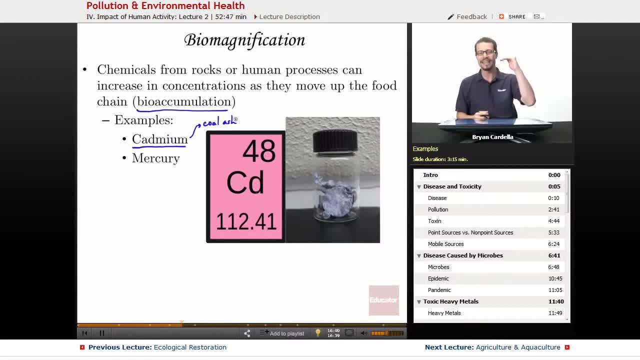 You have insects or other herbivores eating the plants By the time you get up into the carnivores or up into the humans who are eating the animals that have eaten the animals, they've eaten those plants, you can sometimes have 50 times the concentration of cadmium in that individual's. 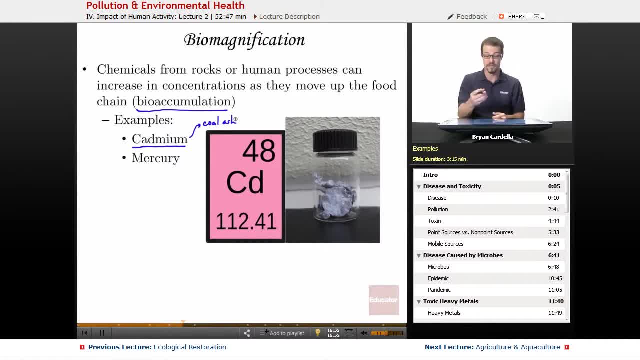 body than what you initially had placed in the soil in terms of what ended up in each individual plant. So if you think about how the food chain works with you know one specific insect, how much plant life they have to eat, and then that animal that eats. 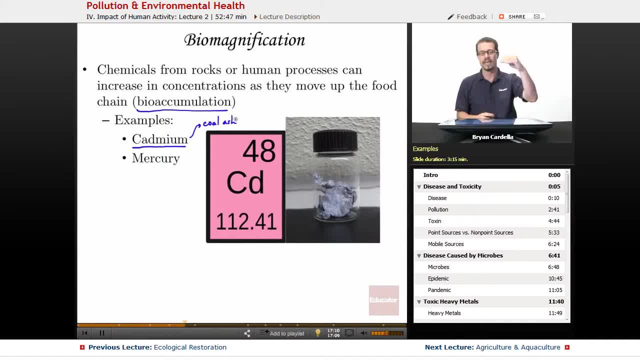 those insects, how many insects they end up eating it can. you can easily see how this bioaccumulation thing can happen With mercury. hey, like I said, it's in the water supply. Human activity especially has put mercury into the oceans. It's amazing that even when you look, 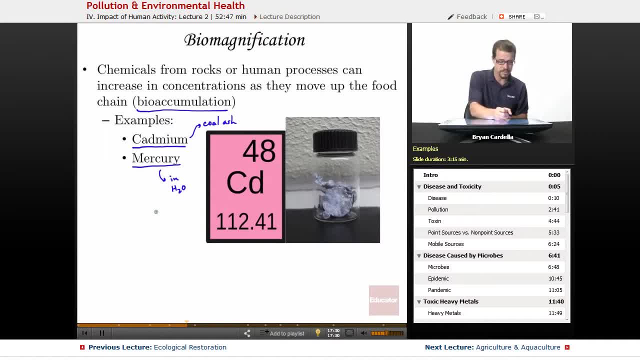 way up in the Arctic Circle where the Inuit people live- oftentimes Inuit populations will be 45 minutes to an hour helicopter ride away from where any civilization exists. So if you want to go visit them, it's quite a trek and they're out in the middle of nowhere, But interestingly enough. 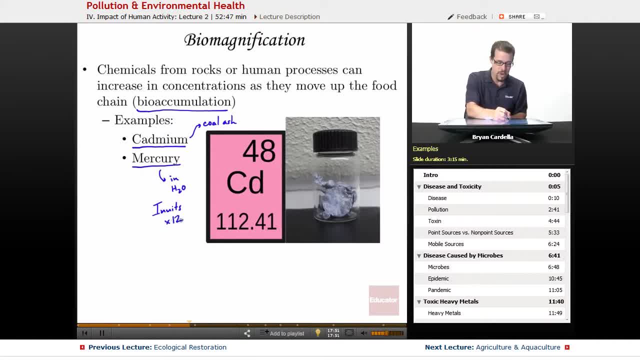 some of these adult Inuit individuals have 12 times the limit of what the United States considers safe levels of mercury in a human body because their diet depends a lot on fish- whale seals- And if you consider that a seal is eating a lot of fish and they're getting an accumulation of mercury in their body. 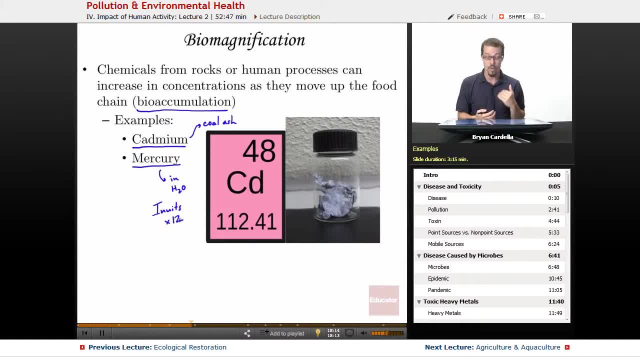 once they eat the flesh of a seal, the mercury exposure is quite great. I've also heard that in Japan, unfortunately, it's fairly commonplace to hunt dolphin and kill dolphin and even sell them on the market. There are some people in Japan who have eaten dolphin meat without even knowing it. 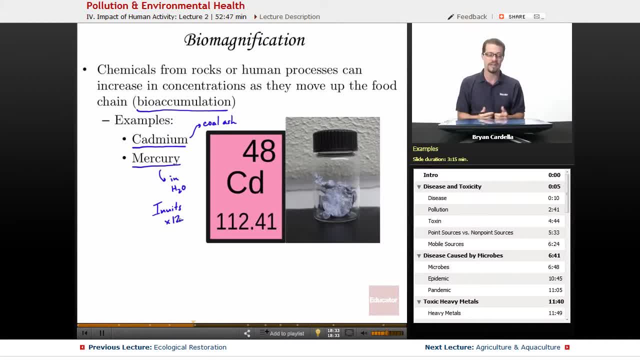 because it's sold and it's mislabeled to make a profit off of it And, unfortunately, if you're eating dolphin meat you're getting a lot of mercury toxicity in your body. Just eating tuna is a certain kind of accepted amount of toxicity in terms of mercury exposure, But imagine eating a dolphin- They've eaten. 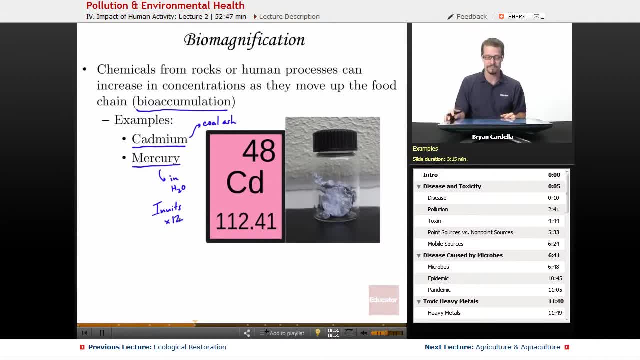 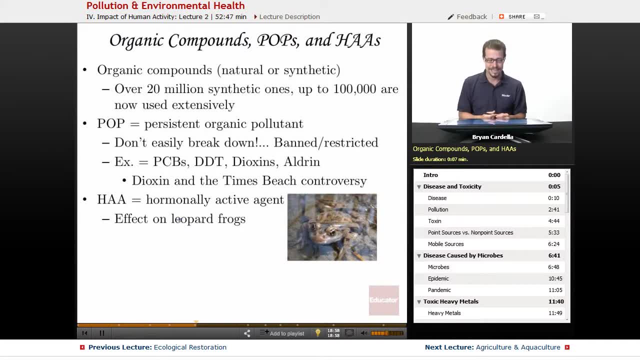 hundreds and hundreds and hundreds of tuna over their lifetime. Organic compounds: POPs and HAAs. pops and haas, All right. So organic compounds: they can be natural or synthetic. Of course there's the natural ones. There's carbohydrates, lipids. 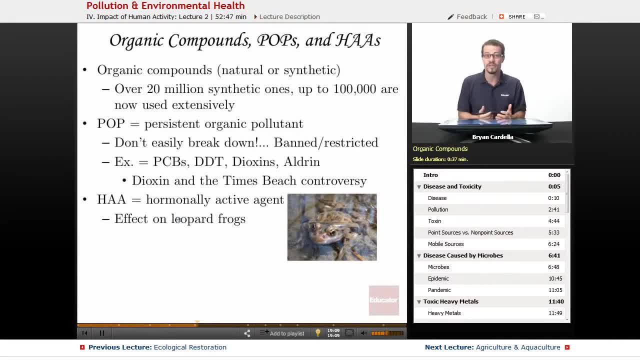 proteins, DNA, RNA, etc. But there's also synthetic ones, the ones made in a lab, And scientists have gotten very creative, especially over the last two decades, in terms of making synthetic compounds. There are over 20 million synthetic organic compounds and up to 100,000. 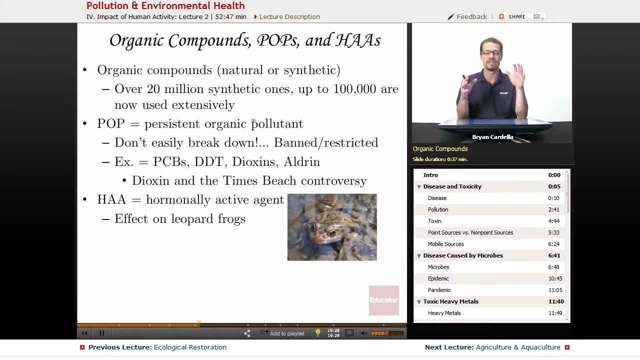 are now used extensively, meaning worldwide, to make all kinds of products, to make drugs etc. 100,000 of them are used quite a bit. What's a POP? Persistent organic pollutant. So it's expected in nature that an organic compound. 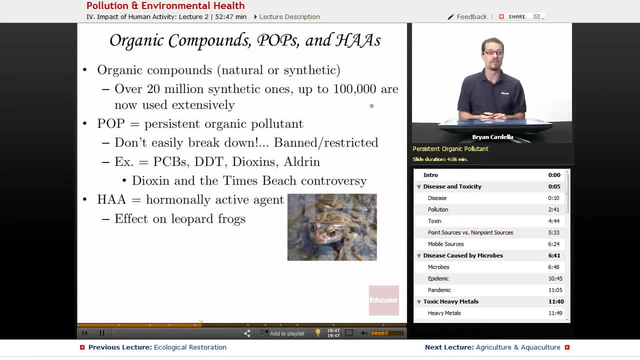 will inevitably be broken down When an organism dies. all of their organic compounds eventually, are broken down by decomposers and end up in the soil, end up in plants, end up in fungi in the soil, etc. And it's just that cycle of energy that we expect, But a persistent organic pollutant. 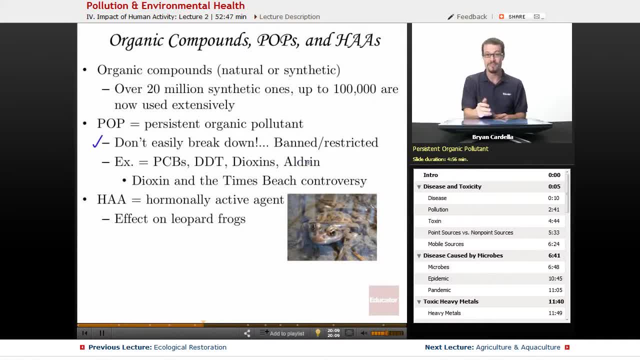 doesn't end up in the soil. It's just that cycle of energy that we expect. It does not easily break down And because of the fact that they just end up in the soil and they end up in the water, staying that way and not being part of this gradual cycle of breakdown, a lot of 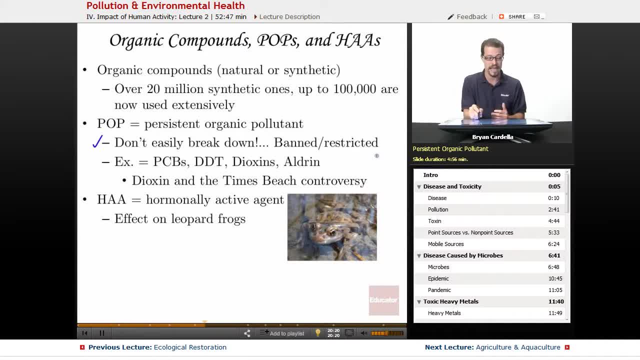 them have been banned or even restricted completely with legal action. So here are some examples: PCBs- PCB stands for- I'll write it out for you- polychlorinated- sorry if it's a little messy- biphenyls. 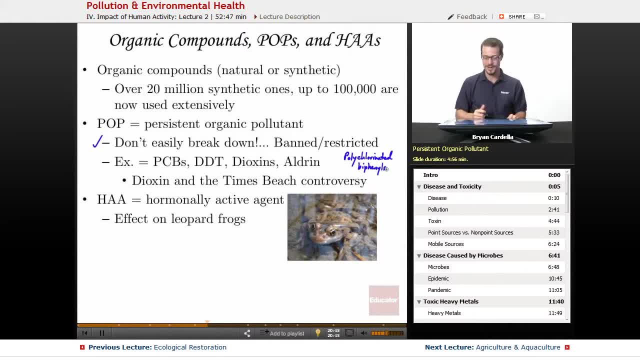 And no, I'm not going to draw them out for you with all those bonds. So polychlorinated biphenyls or PCBs, they are heat-stable oils that have been put in electric transformers. You know electric transformers: there's a lot of heat generated, And so it's an oil that's able to. 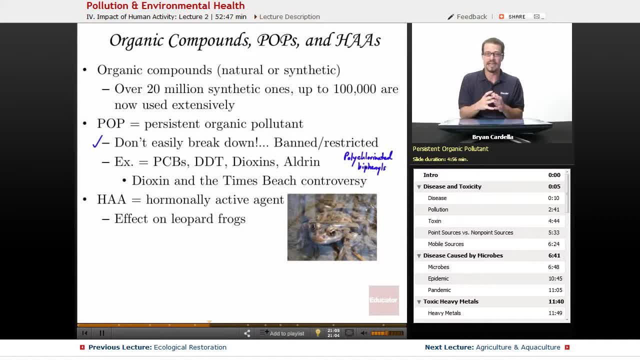 not, you know, light on fire and has like an insulatory capacity. So that's an important thing, right? But PCBs: unfortunately, if something happens with that transformer, if it explodes, if it has a leak, these PCBs ending up in the soil and ending up in the water supply have been known. 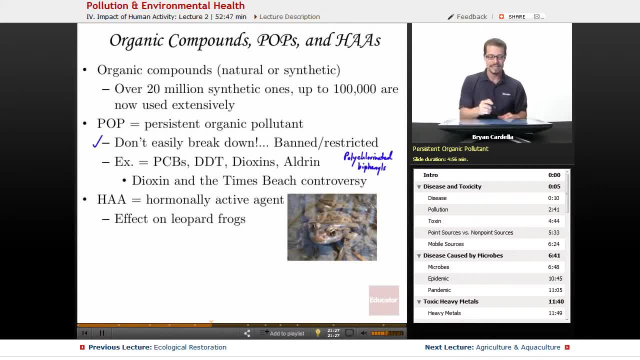 to cause harm. So you know it's a lot of heat generated And so it's an oil that's able to not harmful effects when they end up in the human body- DDT- this has come up before in this lesson. 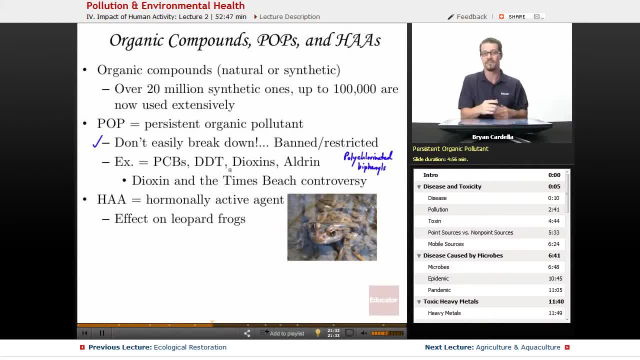 sorry, not this lesson specifically, but in this course. DDT uses a pesticide for many years. Of course, that ending up in humans has caused a lot of problems and in animals, Dioxins. Okay, dioxins is a byproduct of an herbicide, And here's the crazy thing. 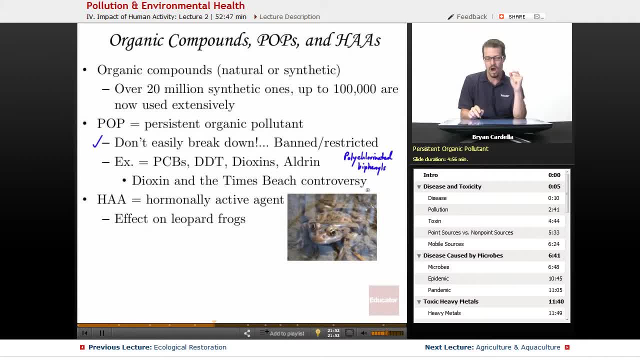 With dioxin, there was this Times Beach controversy. So in Missouri, the city known as Times Beach had used dioxins in a chemical that was sprayed on roads to control the amount of dust. So there were a lot of complaints, maybe even health problems. 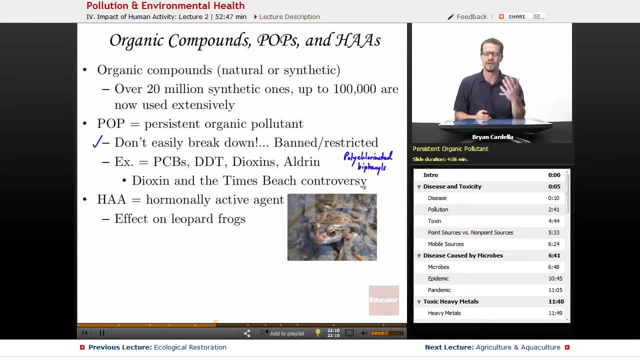 over the amount of dust in the air, People with asthma, et cetera, going to have some issues. So they're spraying this stuff that had dioxin in it. Well, the EPA and other United States organizations came in and they said: you know what The amount of dioxin in the air is going to be? 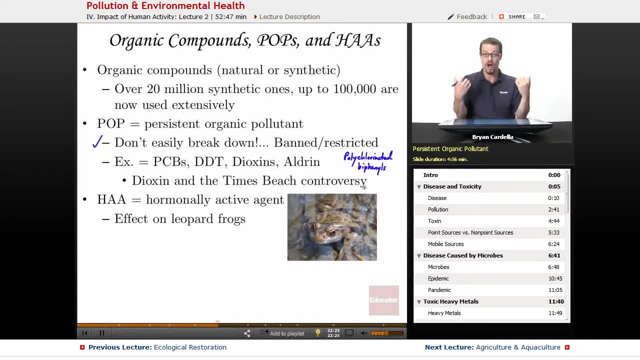 the amount of dioxin in the air, And so they're spraying this stuff that had dioxin in it. Well, the EPA and other United States organizations came in and they said: you know what The amount of dioxin in the air is going to be, the amount of exposure that you've caused with this town. 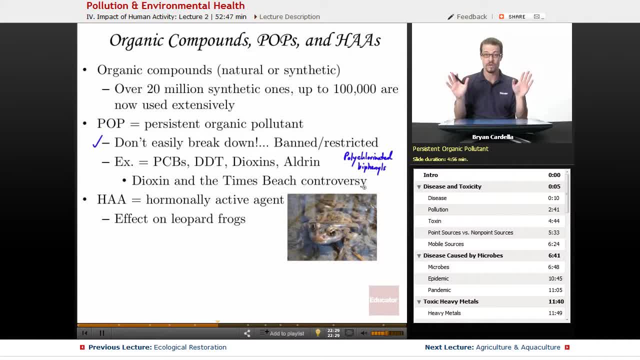 The amount of exposure that these people now have is beyond what we allow. So for $36 million they bought the town. The federal government bought the town, cleared everyone out, So essentially they paid everybody to leave and paid for the property. They bulldozed everything. 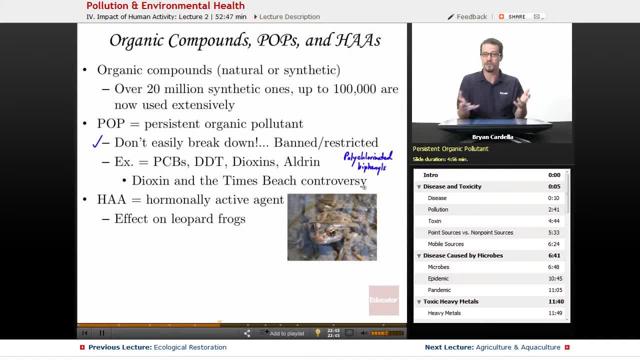 They have now made attempts to kind of set up like this nature preserve in that area And it's gradually coming back in terms of, like you know, the life sprouting up there. but it's no longer in the area, So they're spraying this stuff that had dioxin in it. Well, the EPA and other 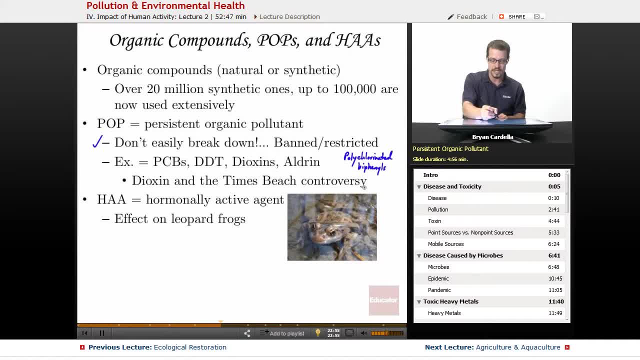 town inhabited by people. It's controversial because with dioxins- here is what the EPA says- is the limit in terms of you know, going beyond this limit is going to cause toxicity in the human body. They say 0.006 picograms, which is 10 to the negative 12th grams per kilogram. 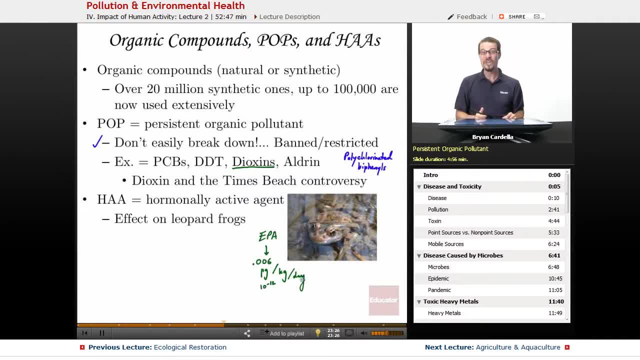 per day. That's really tiny. Even when you calculate that somebody could have, you know, 80 kilograms of mass or 90 kilograms of mass, that's still such a tiny amount. And even one of the individuals who had to do with this uh times beach controversy when 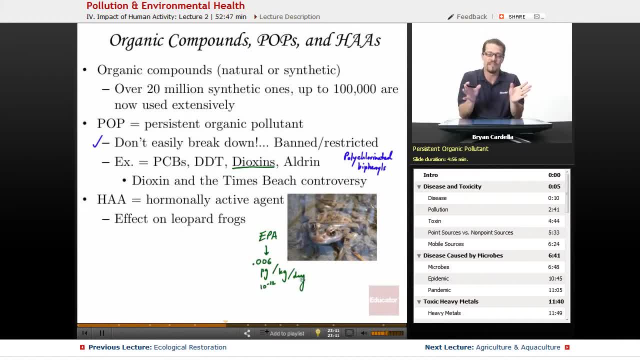 you know, when he actually had a lot to do with making the town leave and and and initiating this. he is now even skeptical, uh, skeptical, of this particular figure. Um, there are some scientists who suggest that this should even be 10 to a hundred times higher than the actual amount. 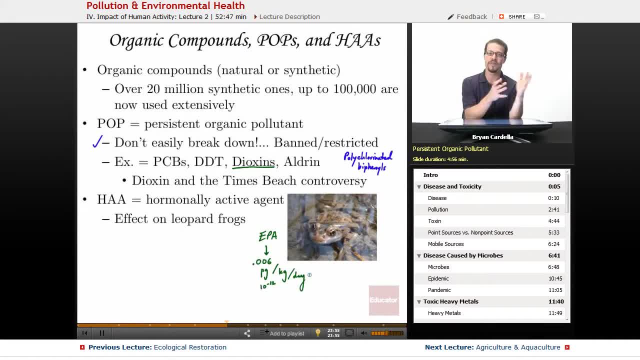 of dioxin in the environment, So, uh, so that's a little bit of a, that's a little bit of a, that's a higher. So that's why it's controversial, because different people have different opinions. The EPA has warned that if we go above this limit, you're going to see negative effects in humans. 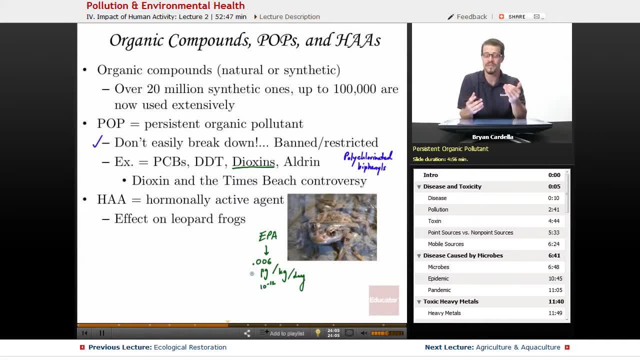 So potentially more studies on lab animals can give us clues about this. but, uh, it's a touchy subject because a lot of people's lives were inconvenienced. but at the same time, uh, you don't want to go too easy on these POPs, these persistent organic pollutants, because, um, you, 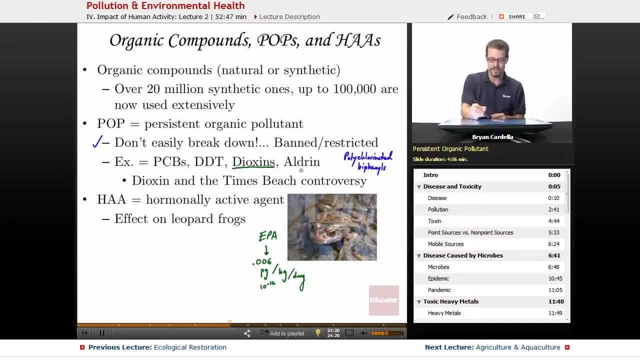 know you don't want people to get sick and or die. Um, Aldrin is another one of those people. who is another one. um, that has ended up in the environment, uh, as an insecticide, and and and caused problems in people in certain doses. An HAA- HAHA is a hormonally active agent, So a. 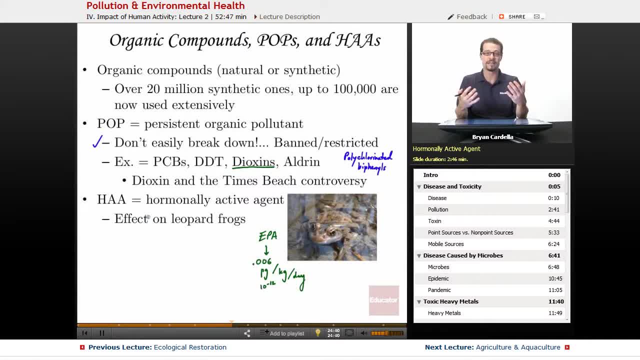 hormonally active agent. it has an effect on individuals' hormones and and the regular or expected uh hormone levels in that person's body, whether they're male or female. So an effect on leopard frogs. Let me give you an example there. There is a chemical called atrazine and it's been 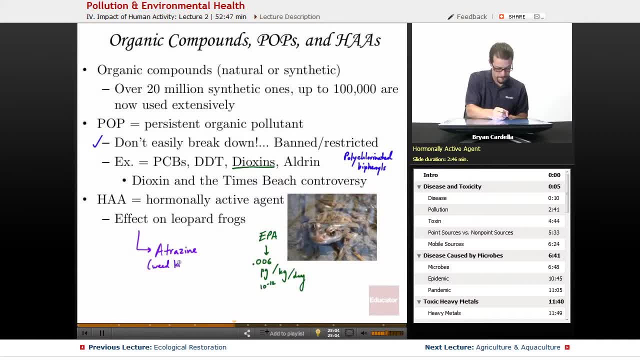 uh used as a weed killer. Well, in Wyoming in the United States, uh, there was a crazy effect that happened on leopard frogs. Here's a leopard frog, a very common species of frog- uh, North America And uh, actually I use leopard frogs oftentimes. 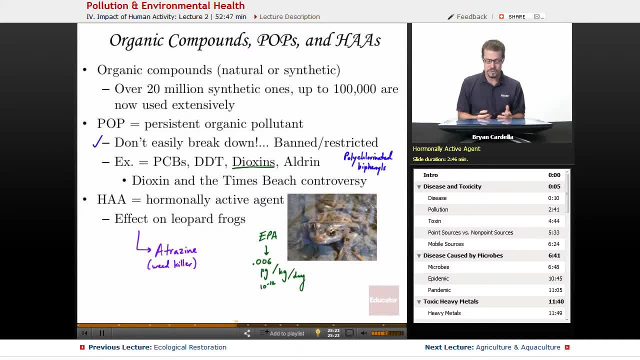 With dissections in biology. But atrazine, uh, as a weed killer, was being used in Colorado And, because of how water moves from the Rockies down into Wyoming, that's how this chemical ended up downstream in this other state And, uh, the amount of atrazine in the water supply ended up. 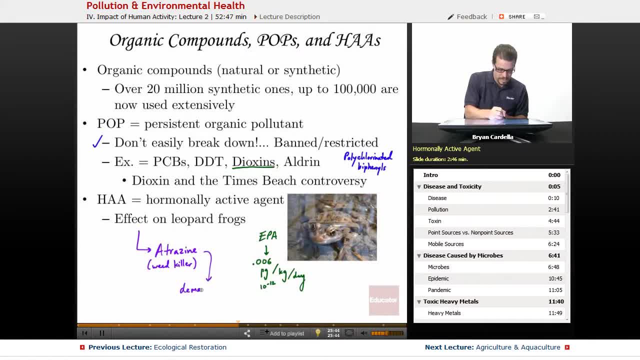 demasculating- Oops, Demasculating- Ended up resulting in the demasculinization- I can't say that Demasculinization, I can't even say that word- Of uh, of male frogs, Basically turning male frogs into females. 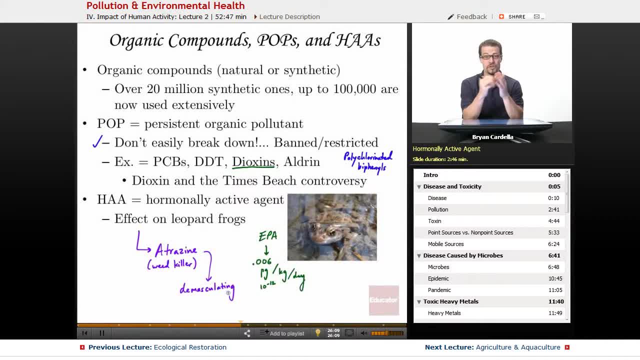 or they also call it the feminization of frogs. So how does that happen? Well, in a male frog, you have a certain genetic exposure due to sex chromosomes. that turns on uh the gonads in order to be testes, in order to make sperm. However, uh atrazine gets in the way of that hormonal. 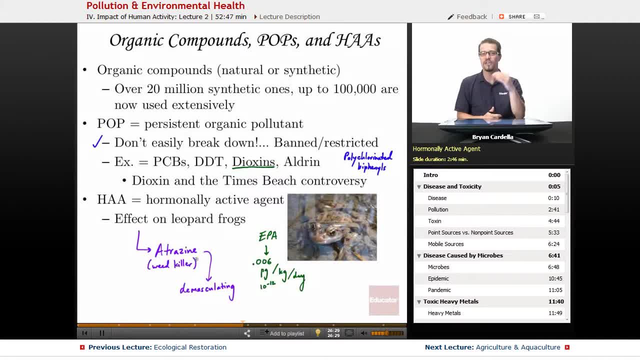 exposure. So the atrazine isn't changing their DNA, It's just getting in the way of the pathway that's supposed to enable the expression uh and the carrying out of that chemical in order to have this sort of uh long-term effect in the frog's body. And so you have a lot of male frogs in. 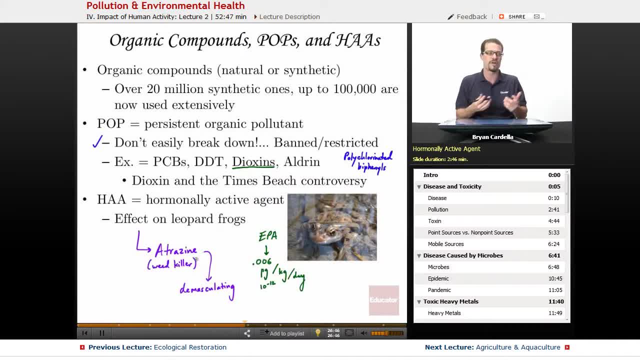 Wyoming, being turned into females. So imagine if, naturally, you end up having close to 50-50 in terms of the amount of atrazine in the water supply. So you have a lot of atrazine in the males and females in a population. If all of a sudden a lot of those males are now turning into 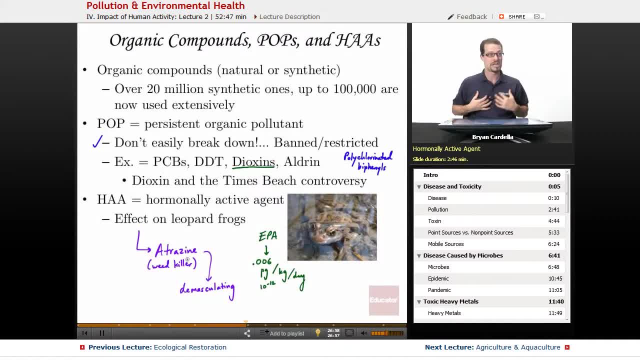 females because of this interference in their- uh, you know- chemical, um, uh triggering in their body. you're going to have a huge reduction in males and not as many offspring, So it can really have a negative impact on a population in a short amount of time. So, keeping track of how we 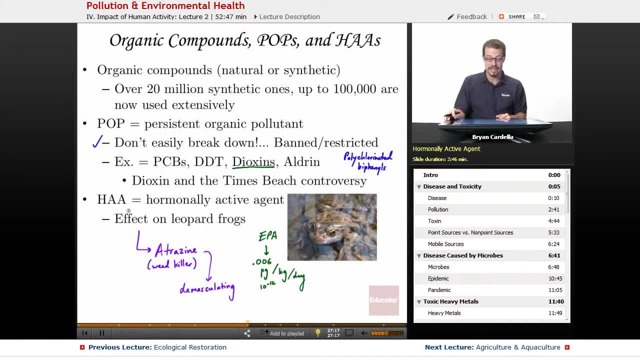 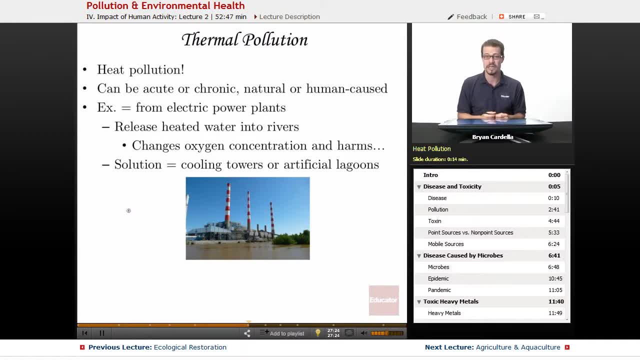 uh, put POPs and HAAs into the environment is a very important thing. Thermal pollution: This is something a lot of people don't think about, but it's heat pollution. Um, this is not talking about global warming. This is talking about, um, typically man-made causes. 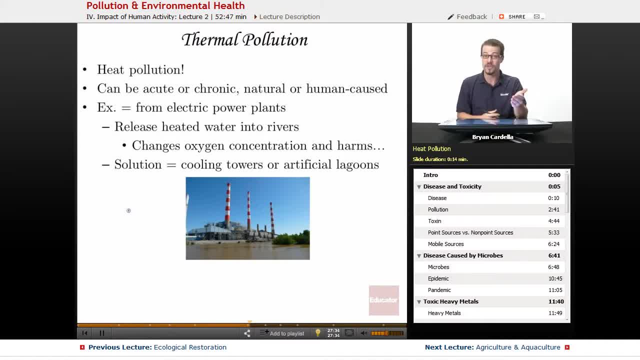 uh in in one area, um like by a factory, for instance, Um thermal pollution can be acute or chronic. So acute meaning uh, short-term, uh, because of you know just a shorter amount of time causing this, this effect, Or chronic, This is long-lasting. 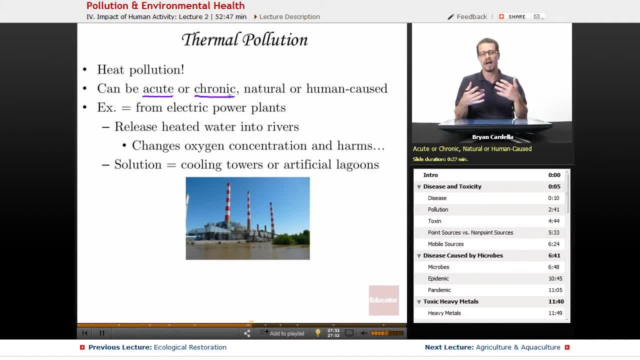 And it can be natural. You can have um changes in the environment that could be considered, uh, thermal pollution, But I'm going to focus on the human-caused kind. Uh, an example is going to be from electric power plants. So release of heated water into rivers, If you've got this electric. 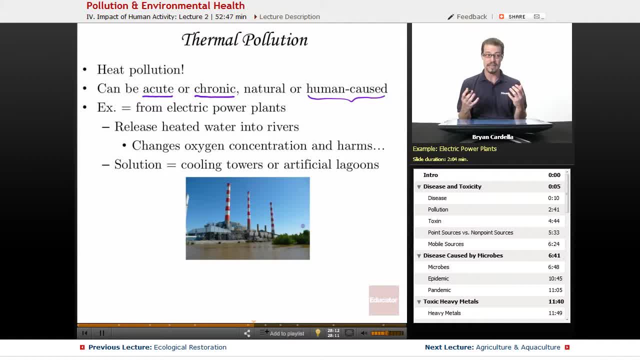 power plant that's generating a lot of heat and as sort of their waste, they're letting out this heated water into nearby river. you might think, oh, what's the big deal? Uh, the animals and the plants. they'll adjust. Not necessarily When you dump a lot of heated water into a river, you're. 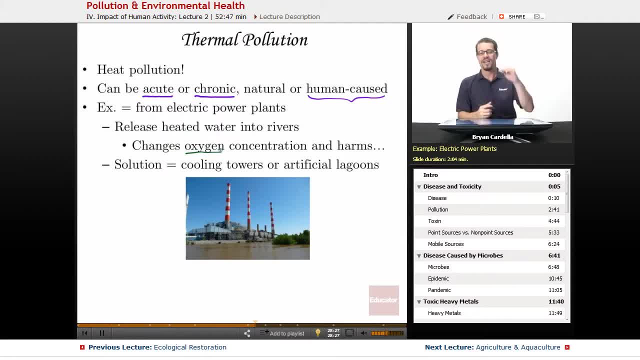 going to have changes in oxygen concentration. The higher temperature of the water, the less oxygen you're going to have dissolved in there. You're actually going to have a lot more of it escaping as vapor, Um, and it harms plant life Sometimes. uh, algae or other plant life are not. 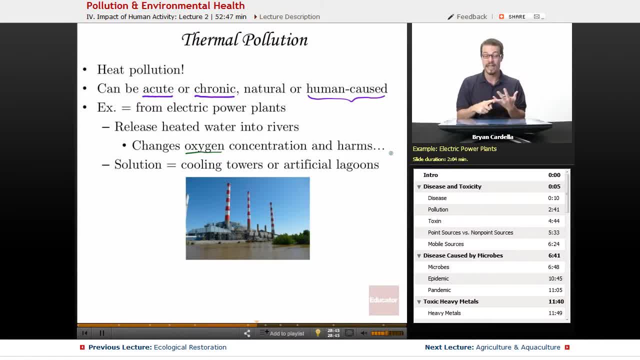 used to that huge change in in heat. Uh, it can also disturb fish, Um, not only, uh, adult fish. sometimes they'll, they'll just swim away, They. they will not be able to stick around, and that can. 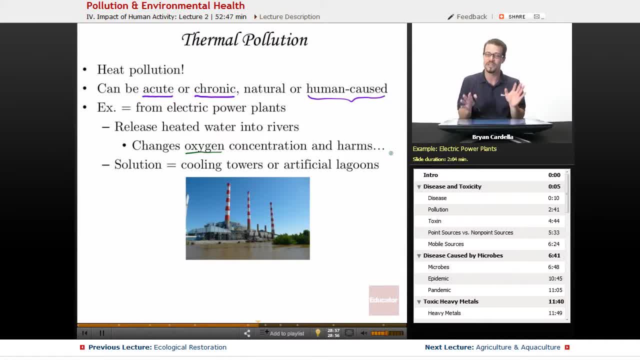 disturb uh, the food webs in the area, But also not just the adult fish, also um the spawning of fish, uh, having their little, you know, fertilized eggs in that area, uh, they have a certain. 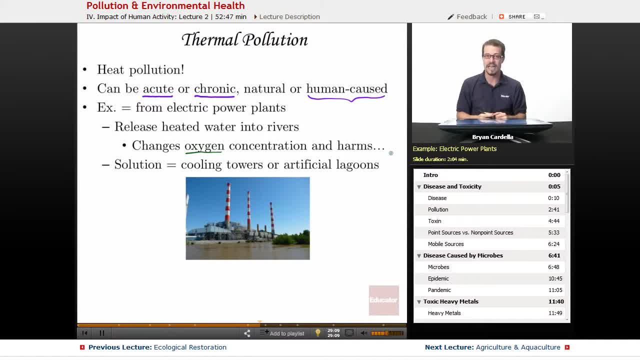 temperature range that they have evolved to exist in. And if we have this short-term change over the existence of this electric power plant, where you have huge increases to the the degree of temperature in that water, um, you could have the fish population just being damaged um to the point where it can't be. 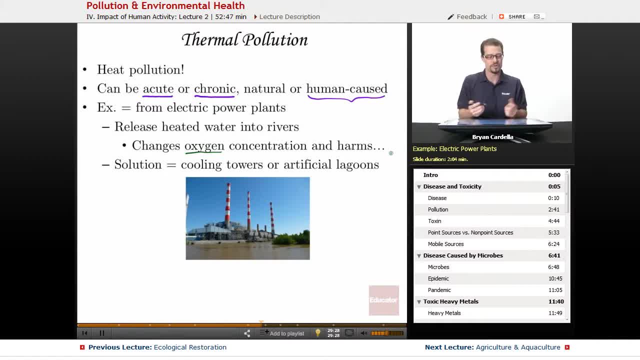 repaired. So solution: how do we uh deal with this? thermal pollution- Cooling towers. Some factories have done the responsible thing and installed a cooling tower where they put the heated water in this area. that allows it to be cooled to a acceptable, more natural temperature. 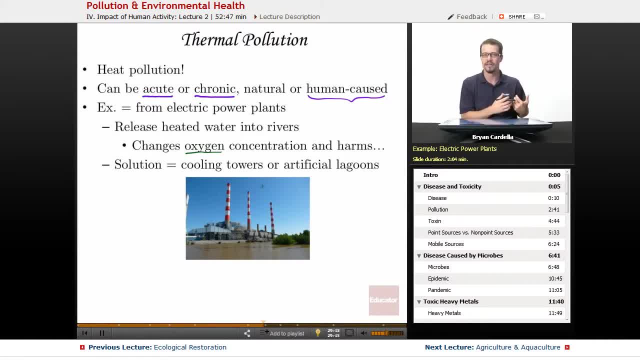 that matches the surrounding environment, And then it's it's disposed of in the environment Or artificial lagoons. So if you can put the heated water into this man-made lagoon like a little mini lake, temporarily, let it cool down and then, once it reaches an acceptable temperature, you let the uh, the gates open and it goes into the river. 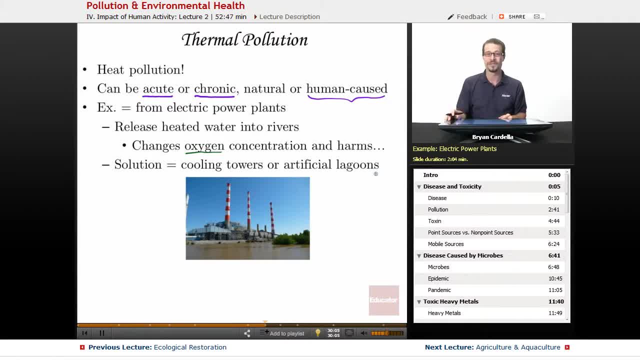 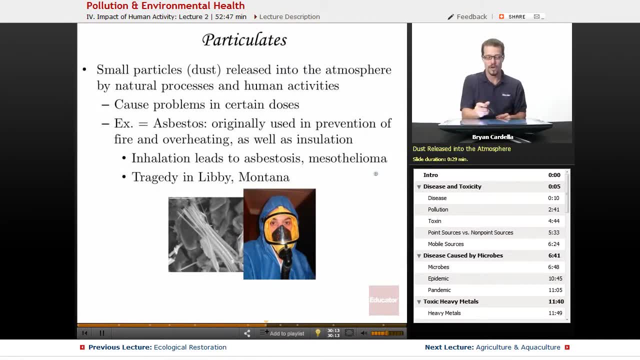 So those are some solutions for thermal pollution. The pollution solution: Particulates. So these are small particles, also known as dust, released into the atmosphere by natural processes and human activities. more on the human activity side of it, They cause problems in certain doses. So you and I may have. 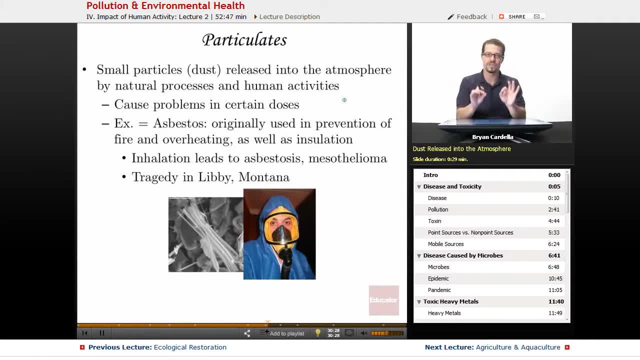 been exposed to a lot of these particulates, but the dose was so tiny that there are no noticeable effects. We have not reached past that threshold of what's considered dangerous. An example- the classic example- is asbestos. Asbestos originally used in prevention of fire and 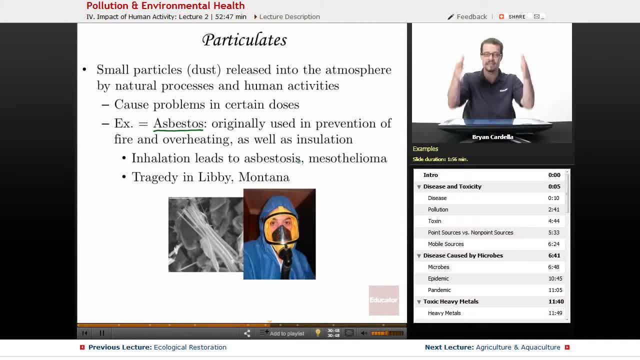 overheating as well as insulation. So inside of the walls of an apartment building or a house or some other complex, Usually if there's a really old building and they're going to be doing stripping of the walls and tearing down of layers, if the person who's heading the project knows. 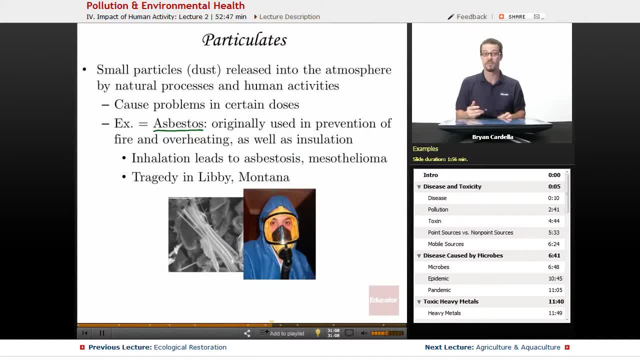 hey, asbestos was used in this building. they will go in with these masks to protect themselves. You do not want to be inhaling asbestos because in certain doses the inhalation leads to asbestosis, which is basically an infection due to asbestos exposure in the lungs. 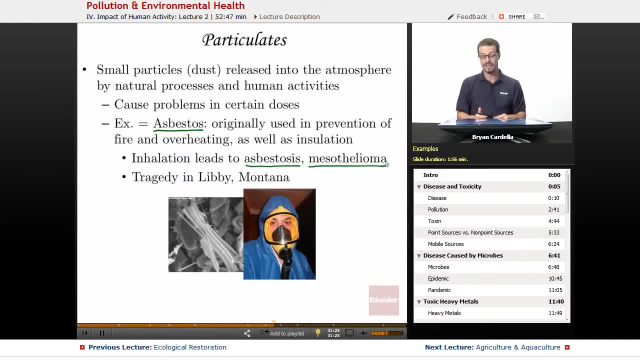 or mesothelioma, a chronic illness as a result of asbestos exposure, And lung cancer too. Just a lot of different problems can be caused by this, And actually I've seen commercials where there are class action lawsuits. If enough people in a workplace 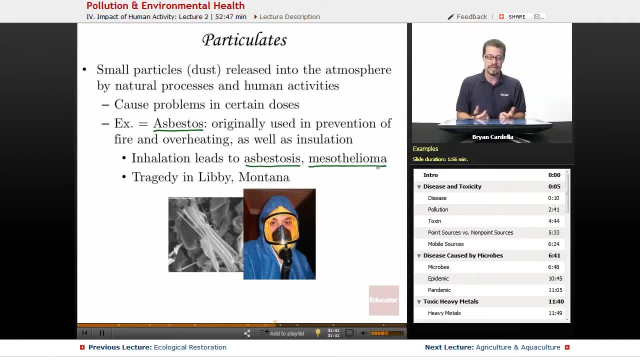 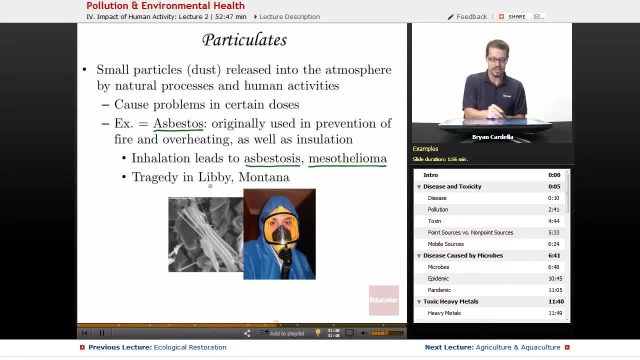 These cases have gone to court. There was a tragedy in Libby, Montana, over asbestos, So workers in a certain area knew that there was asbestos exposure and they were wearing masks, However the asbestos getting onto their clothing and onto the things they would take to and from work. 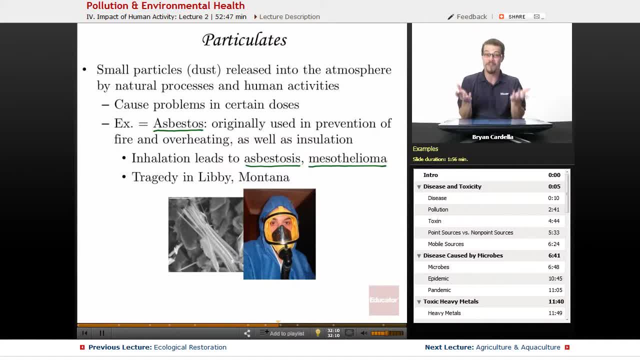 every time they would go home, they would gradually expose their families to those particular particulates And a lot of people got sick. A lot of people have gotten these chronic illnesses as a result. And it's just this stuff here. This is a microscopic view of what these fibers look like. 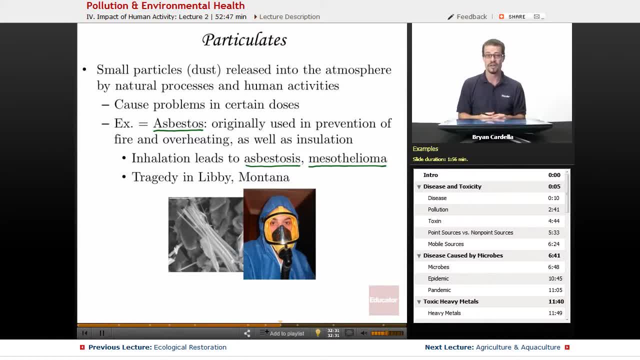 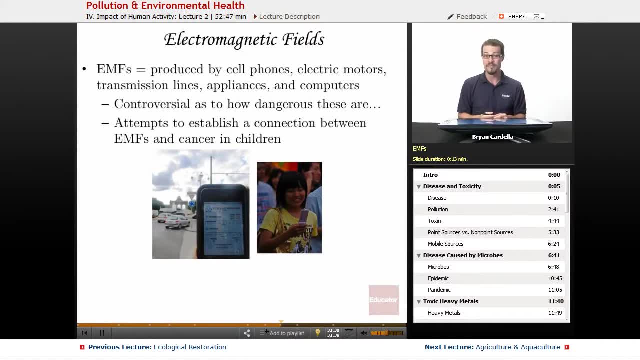 And enough of them, introduced into the lungs, cause really severe lung damage. So it's not to be trifled with Electromagnetic fields, also known as EMFs for short, produced by really anything electronic that you own- cell phones, electric motors, transmission lines, appliances, computers- and it's controversial as to how dangerous these are. 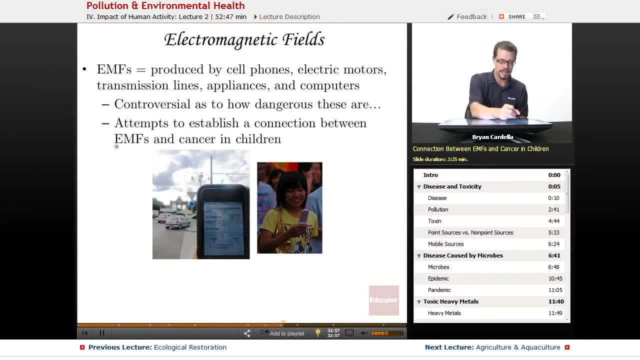 There have been attempts to establish a connection between EMFs- electromagnetic fields- and cancer in children. This is very controversial, So whether it's using this little guy here or this girl using her cell phone, there have been studies confirming that. There have been studies confirming that. 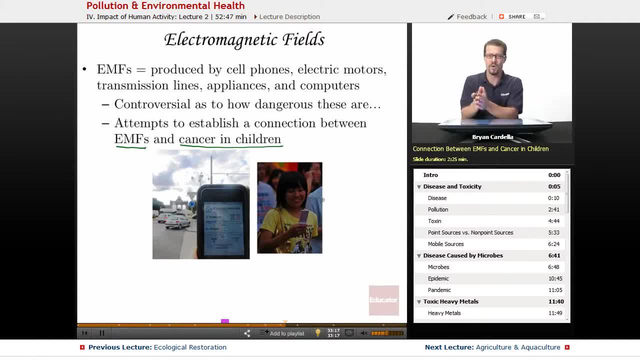 There have been studies confirming that There is a link that children who live closer to power lines, closer to power plants, closer to areas where there's a higher degree of these EMF exposures, that their chances of developing cancer are slightly higher than other children. 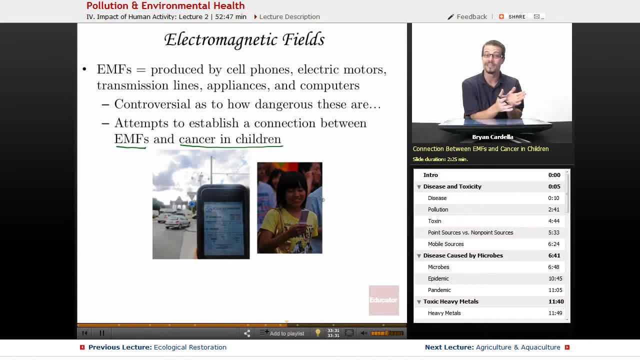 However, there have been other studies that have confirmed the exact opposite, that they have no greater chance than children living in a rural area where there's a lot less EMFs. So the jury is still out on this. That's the expression. As time goes on, I think scientists will get better. 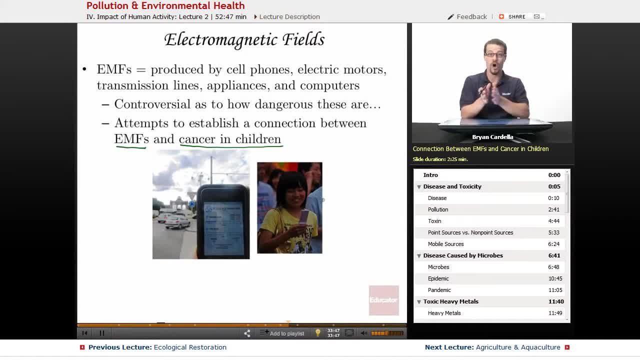 It's separating the EMF factor from all the other factors in that person's life. For instance, with the study that confirmed that there was a higher rate of cancer with EMF exposure versus the kids who were far away, there may have been other factors that those children in that neighborhood shared besides the EMF exposure. 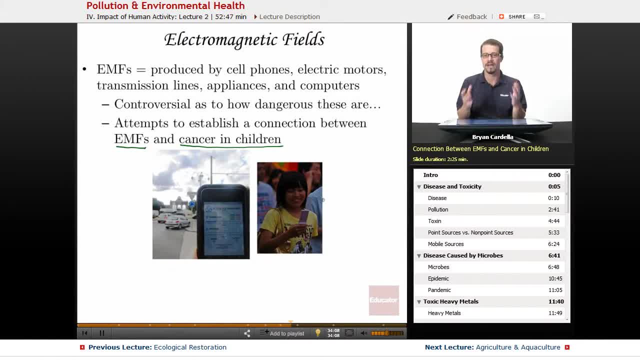 whether it's something in their diet, hormone exposure, whatever it might be, you know if it's an HAA. So as time goes on, we'll know more. There have been theories that increased cell phone use is likely to cause higher cancer rates in the near future. 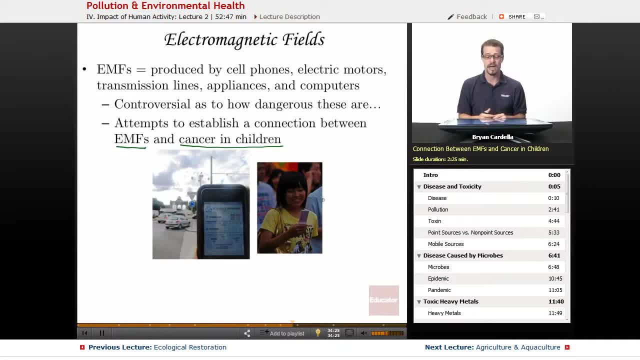 This is just a theory. This has not been substantiated yet and we'll see if there are studies that do make a solid connection with the scientific method. I've also heard theories that perhaps increased EMFs in the last few decades have had an effect on bees. 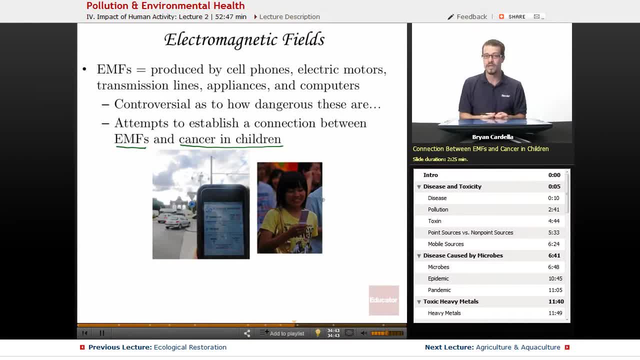 So I've talked a little bit about the colony collapse disorder. in this particular course I had a conversation with my friend who's also a scientist. His theory has a lot to do with genetic modification of crops having a negative effect on the bees. 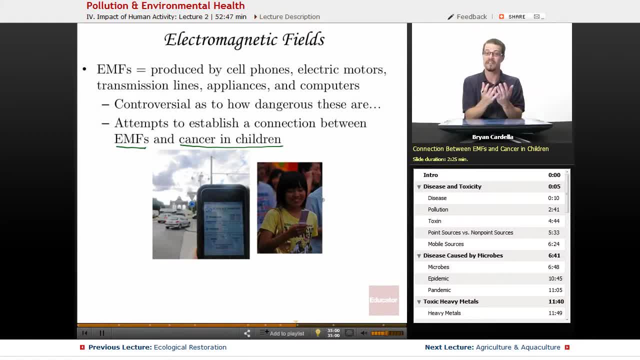 I think it may be a synergistic effect, some kind of combined effect where changes to crops over time- and the bees do rely on plants and we've affected them- combined with EMFs may have these detrimental effects on hives and we'll see. We need more studies on how EMFs affect us and other organisms. 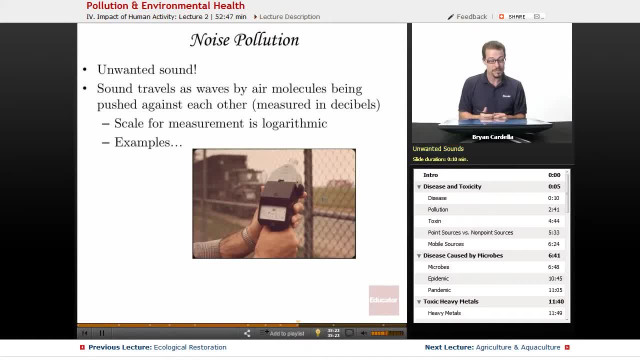 Noise pollution. You don't hear about this a lot. Noise pollution is unwanted sound. That's certainly subjective, right? If it's unwanted, it means that certain people don't want it, or maybe all people don't want it. Sound travels as waves, So this is something you learn about in physics. just a general you know science concept: Sound travels as waves, not as 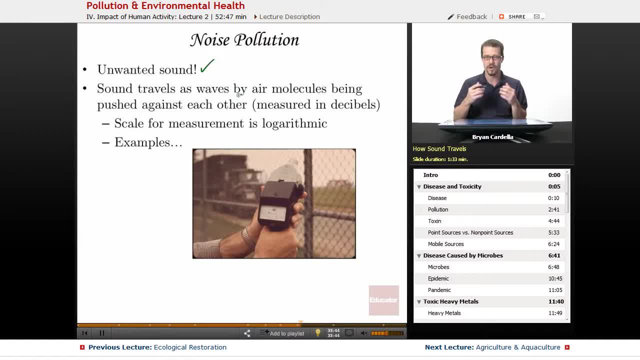 electromagnetic radiation as with like visible light or x-rays or something like that. No, These are waves that are usually represented by this symbol, rather than you know waves that look like that. So this symbol here it kind of looks like the volume increasing on an electronic device like your computer. 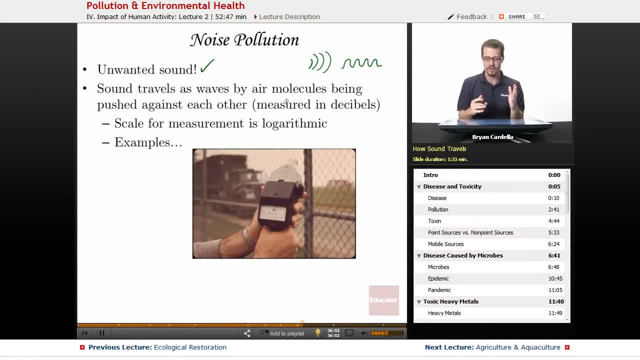 but it's air molecules being brushed up against each other. So the vibrations, in terms of how they brush up against each other, determines how high-pitched or low-pitched the noise is: The the amplitude in terms of how loud it is. 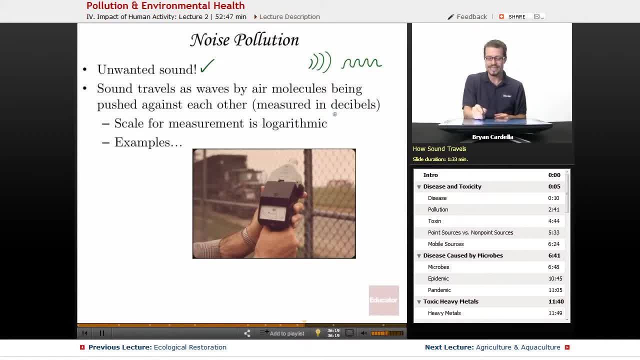 the force with which they're brushing up against each other, and it's measured in decibels. Okay, so decibels dBs is our unit for for sound, And the scale for this measurement is logarithmic. Here's what that means: If you had a sound that is 10, 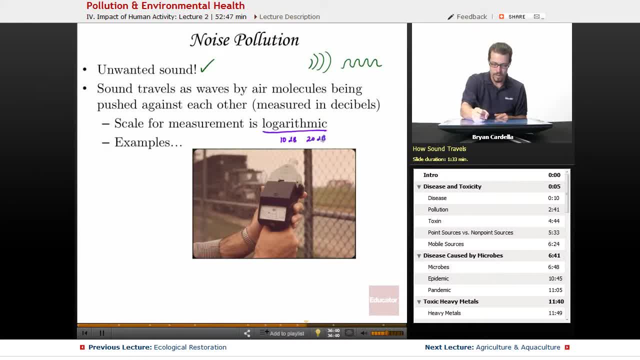 decibels and then a sound that is 20 decibels. well, the 20 decibel sound is 10 times as strong as the 10 decibels, So that makes sense. It's literally 10 decibels louder, But when you get to 30 decibels, 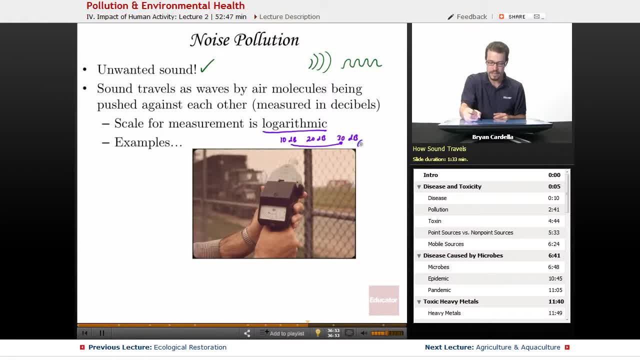 from here to here, it's actually a hundred times louder. Then when you go to 40 decibels, that's a thousand times louder than 10, and so on and so forth. So that's why it's logarithmic. So we're talking about an incredible range. 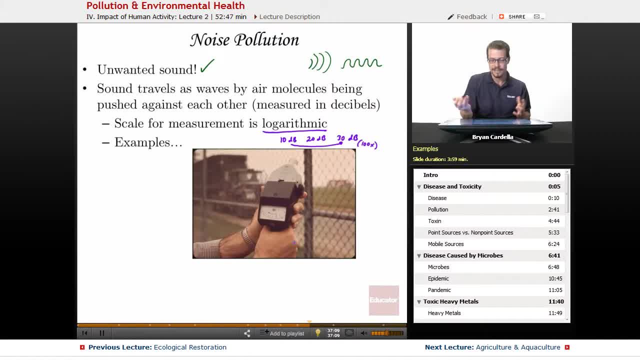 Let me give you some examples. And, by the way, if you're wondering what the heck is this? it's, it's a decibel meter. It's it's used to measure. It's a decibel meter. It's, it's used to measure. 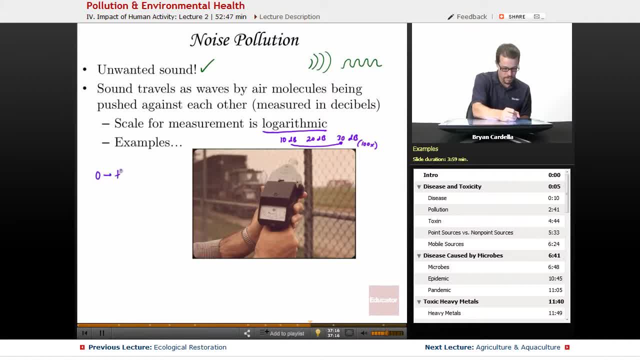 It's used to measure sound. All right, Zero decibels, That's the threshold Meaning. you may not be able to distinguish a zero decibel sound. That's really what it's pointing at, That below zero you can't hear any of it, the average human at least. Once we go above zero. 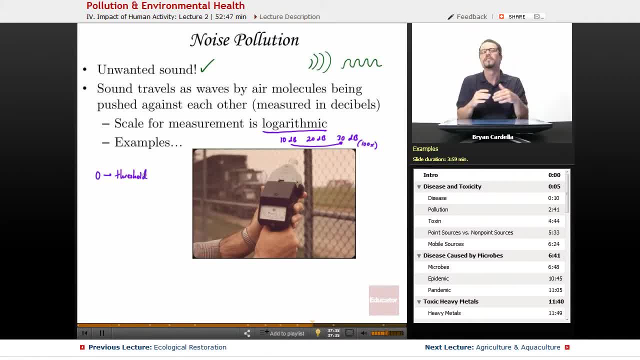 Oh, I think I just heard something. It was very faint. So when you get finally to, like you know, five or ten, you can actually hear it. 20 decibels is a is a whisper. Hey, this is about 20 decibels. 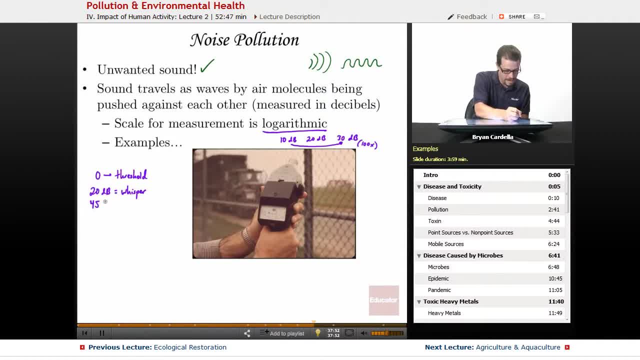 Can you hear me? I'm 45.. I'm going to use the ditto mark for decibels. That's the average home. So if you are sitting in your home or apartment by yourself not making any noise, There's still noises around you. 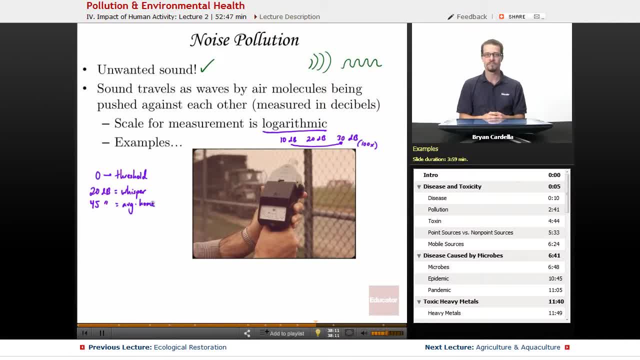 Like when I sit perfectly still in here and don't allow my chair to creak. i can actually hear the computer off to my right. i can hear it humming. it's very, very faint, but there's noises that happen, whether it's your refrigerator, your dishwasher. the hum of, however. 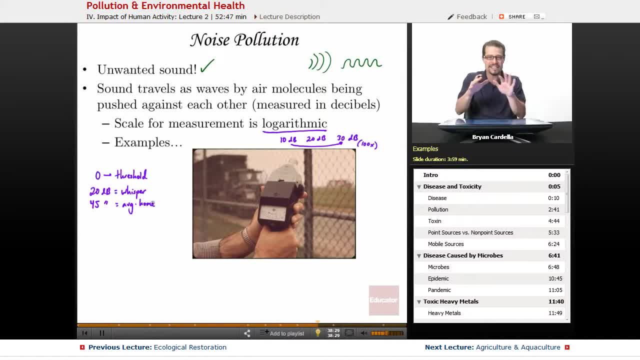 you get ac into your place. the average home has a sound 65 normal conversation, a norm convo kind of my. i actually talk a little bit louder than the average person, but right about here, this is: this is a normal conversation. this is about 65 decibels. 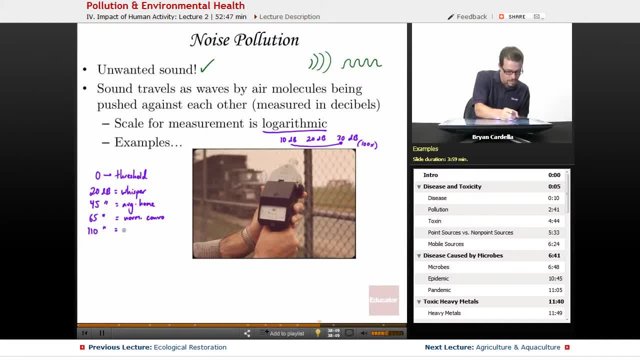 uh, 110 decibels rock and roll rock concert. uh, so yeah, when i saw pearl jam last year, um, it was pretty loud and i enjoyed myself, but i probably should have brought earplugs. i've actually, uh, read accounts by pete townsend, the guitarist from the who classic rock band. 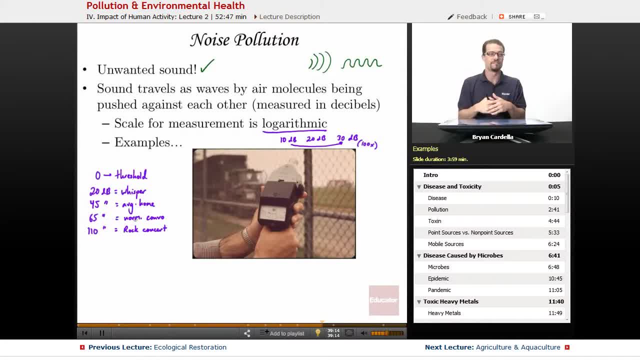 he has permanent hearing loss because of so much guitar playing over his many years. you know his just about 50 years of being a famous rock musician. uh yeah, he now warns the youth like hey, you guys are even listening louder, louder and louder to your. you know personal. 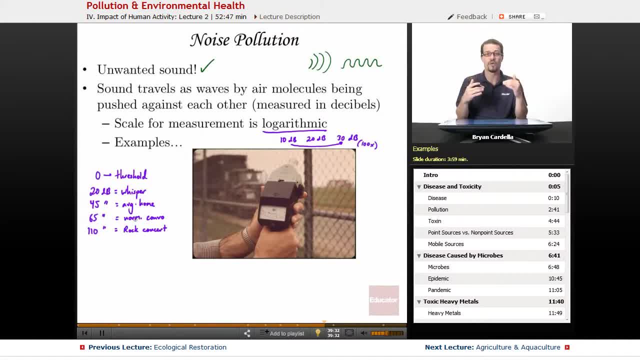 music than i did when i was a child, and you know people go to a lot of concerts or play a lot of music. they're at risk for permanent hearing damage. so wearing those ear plugs actually be something that's wise to do. you can still hear the music. it's just a little muffled and then of 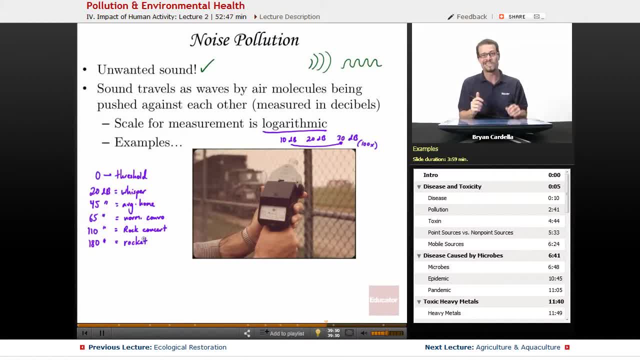 course, once you get above about 160, you're talking very immediate hearing damage: a rocket launch, rocket launch at 180. so and if a plane takes off, we're talking, you know, 165, 170. uh, you need those huge industrial like- oh i can't hear what you're saying- kind of headphones, because 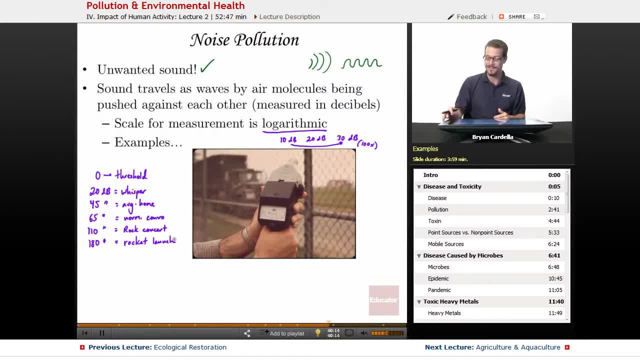 yeah, that's a massive, massive sound wave going into your ear hole. oh, besides noise pollution, there are other forms: light pollution. that's something a lot of people don't think about, but i live in los angeles. there's quite a bit of light pollution, to the point where 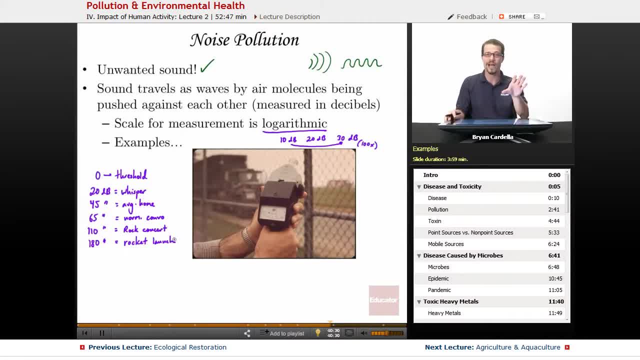 i can't see the stars very well, so going camping, you know, a couple hours out of la very nice, for seeing the stars in the milky way. light pollution has also affected organisms like sea turtle. uh, when sea turtles hatch, they naturally, instinctively, want to go towards the water. 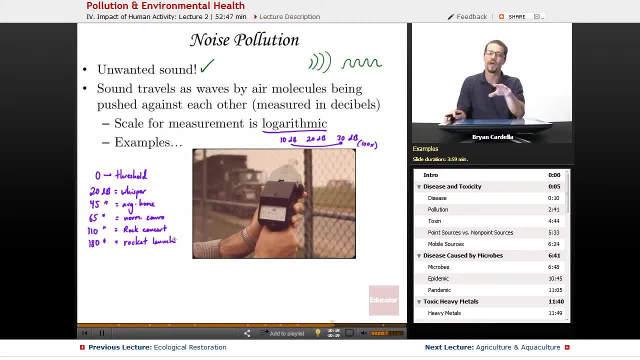 and they kind of will see like the moonlight reflecting off the water and go that way. but unfortunately some sea turtles have been attracted to lights of the city that are away from the water and some people might think, well, those are stupid sea turtles. no, that's a human. 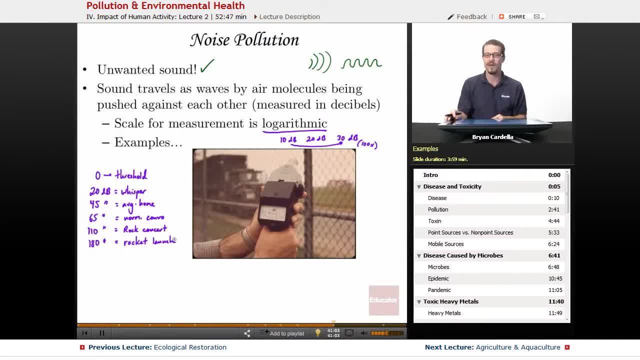 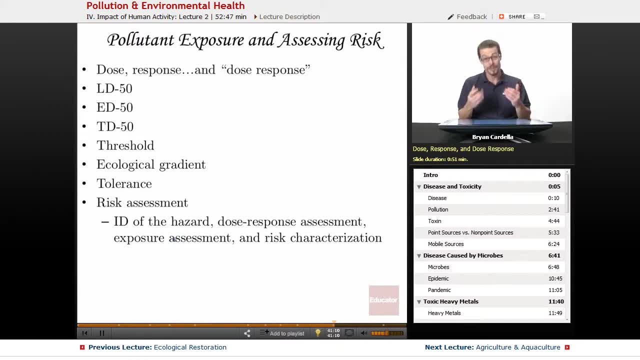 activity that has negatively impacted that species. it's something you don't think about that often. all right, pollutant exposure and assessing risk, dose response and dose response. so a dose is the amount that an individual is given, right? if you're on a medication, you take a certain dose certain number of times a day. 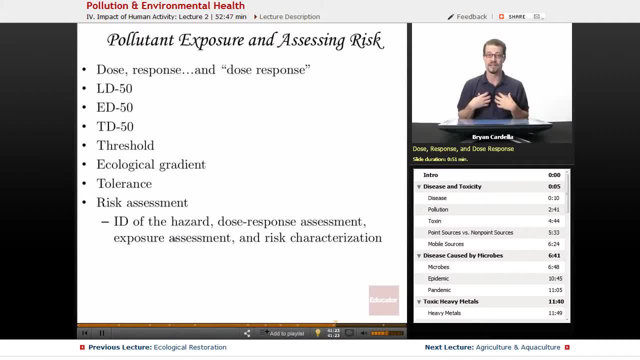 certain times per week, etc. the response is the effect on the body. now, dose response is those two things together in terms of how a human is affected by this particular pollutant or this drug. so, whether we're talking about a pollutant or drug, i'm actually using certain drugs and i'm not going to go into all the details, but i'm just going to 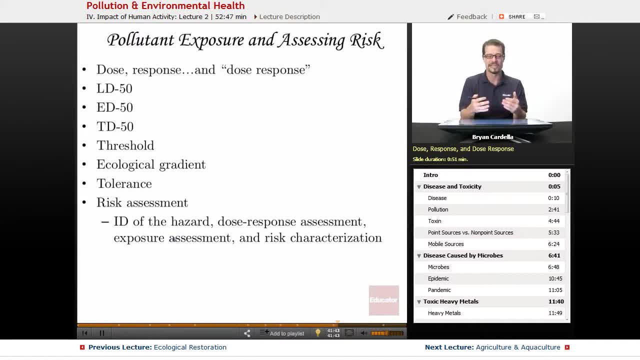 give you a little bit of an example of how a human is affected by certain drugs or certain chemicals. you don't consider pollutants as an example in this particular slide, but when you're talking about this stuff you're going to see ld, ed and td50 depictions in terms of kind of a linear graph. 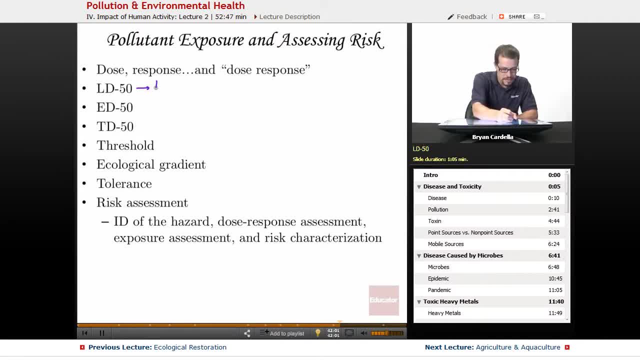 in terms of how people are affected. so here we go with ld50. this is lethal dose for 50 percent a population of people or animals, a study group, whatever the group is we're talking about. the lethal dose means 50 percent of the population dies at this level. so with ld50, um, you're not. 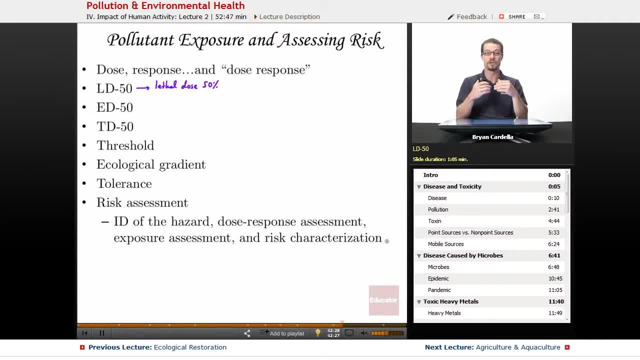 going to see a lot of those scenarios when you're when you're testing a drug or pollutant on people. we don't want 50 of people to die. that's inhumane, that's terrible. but you'll see ld50 if they're testing a certain drug in the initial trial. you're going to see a lot of people die in the initial trial. 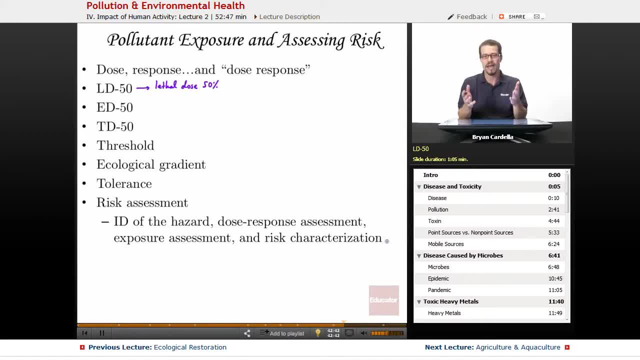 on lab rats and i know whatever lab animals use. i know a lot of people out there are opposed to that, but some of the benefits of using those animals is undeniable. so, um, unfortunately, yeah, there are cases where in the initial trials, hey, 50 of them died. we want to shoot for a dose that. 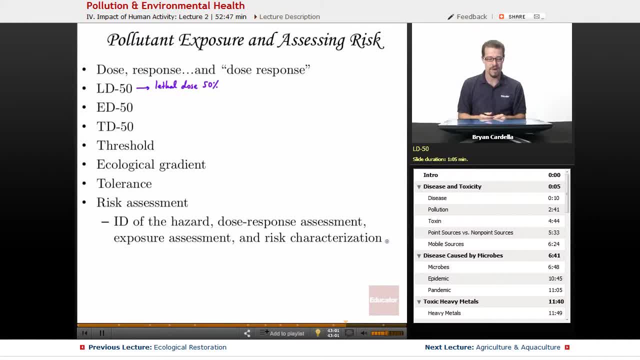 is lower than that. obviously, if that dose killed half the population- ed50- this is the effective dose for 50. meaning at this level, at this dose, 50 of the group- there is an effect that is noticeable, that's tangible, you can see it. um, let's say we're doing a study on aspirin. whatever dose cures the. 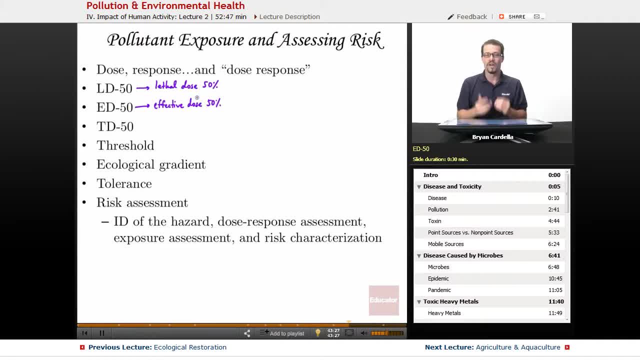 headache. in 50 of the people, that's the ed50, and then td50- this is toxic dose, and then td50- this is toxic dose, and 50, so not enough to kill the individual, but it's a toxic level. uh, so you're getting past a. 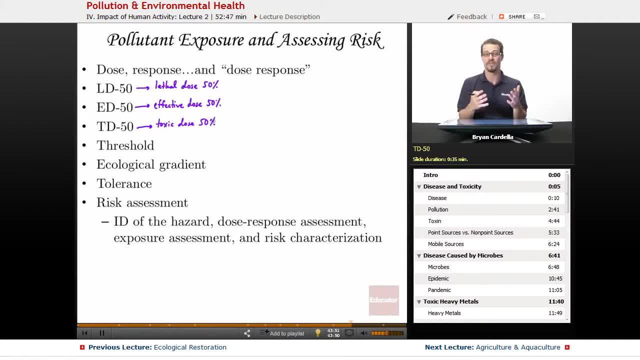 threshold where now there are these negative health effects. so this could be like the: the pollutant or drug has interfered with enzyme activity. um, you're getting uh severe negative health effects. the individual has not died, but you're talking long-term negative health effects. uh, at that toxic dose level. 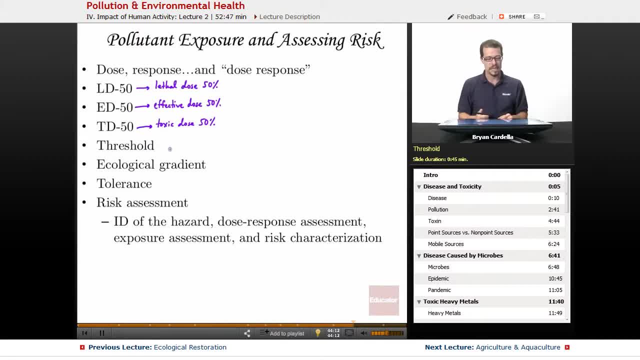 all right, threshold, i mentioned this earlier in the lesson. threshold, uh, we're talking about below that level. there's no noticeable change in the individual. but above that level, above the threshold, you start to see either an effective dose- hey, it's starting to affect them. oh, toxic. 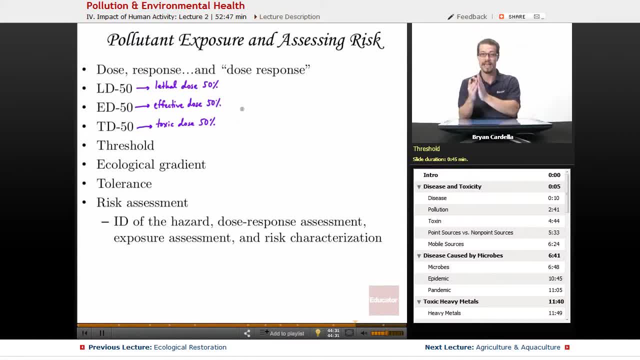 and then lethal. if we were to order these in terms of like, hey, here's the one, then the other, than the next. first you're going to see the effective dose, hopefully like, oh, we're starting an effect on this individual. then you get to the point where it's td50: oh, 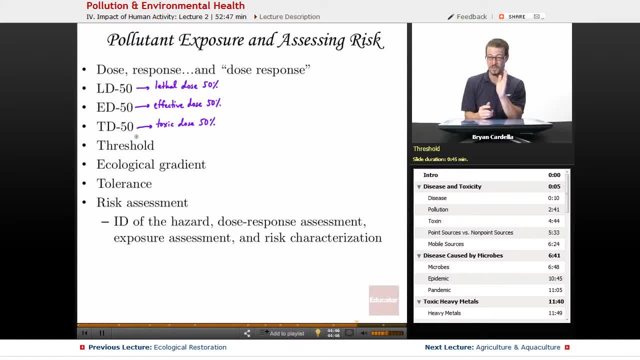 now it's. now it's toxic. now there's these negative health effects because we've exposed them too much and then after that it's typically going to be lethal where, at that level, then 50 of them are dying. an ecological gradient is an interesting application in environmental science with 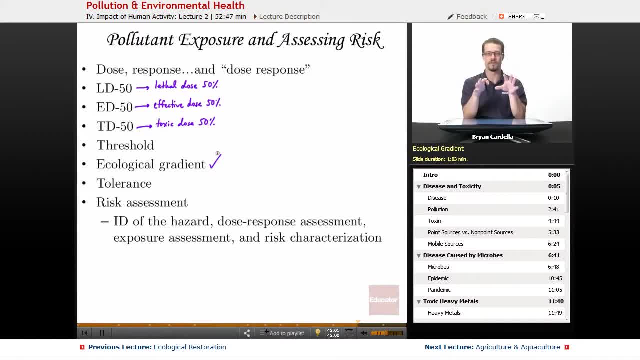 pollutant exposure. if you have pollutant exposure from, let's say, a point source, certain factory, smokestacks, whatever the ecological gradient is when you see how life is affected moving away from the factory, oftentimes if there's a lot of that pollutant nearby the factory, which makes sense because it's close to the point source, you're going to see. 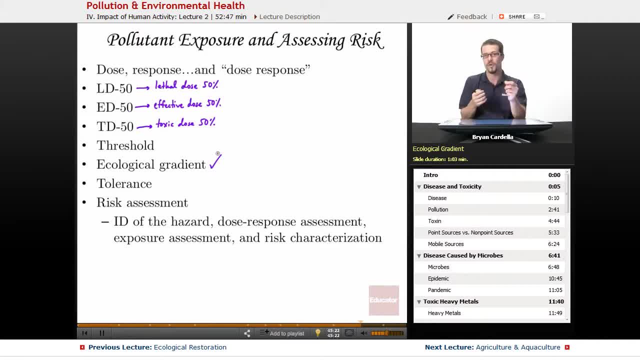 a lot less trees. maybe there's only certain weeds growing there and certain plants that have tolerance to like toxicity levels and they grow quickly. whatever might be, and as you move farther and farther away, you're able to see a wider variety of plants, because they're farther away. 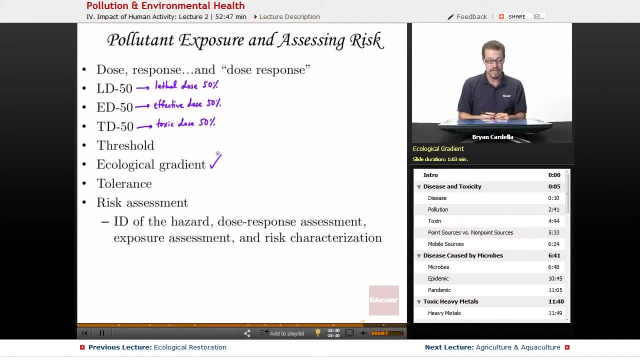 from that pollutant and there's less exposure. so that's an ecological gradient and you could also see the same in human populations in terms of how close they are to a pollutant. there certainly was an ecological gradient with the chernobyl nuclear disaster and you're going to see more about nuclear power in a 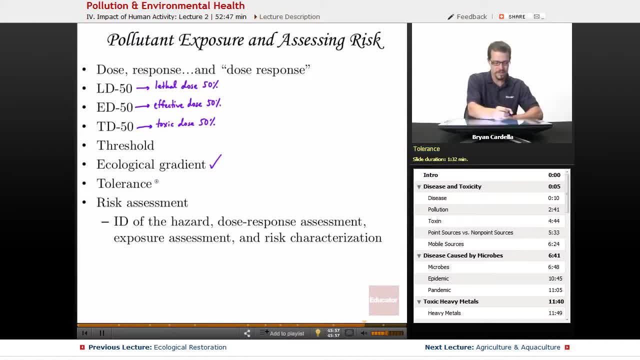 future lesson in this course: tolerance. there are different forms of tolerance. you can have physiological tolerance. an example is ozone, o3. so oxygen gas is o2. that's normal and useful for us to inhale, that we need that as a aerobic organisms. but o3- you normally wouldn't be exposed to. a lot of that. o3 ozone is found. 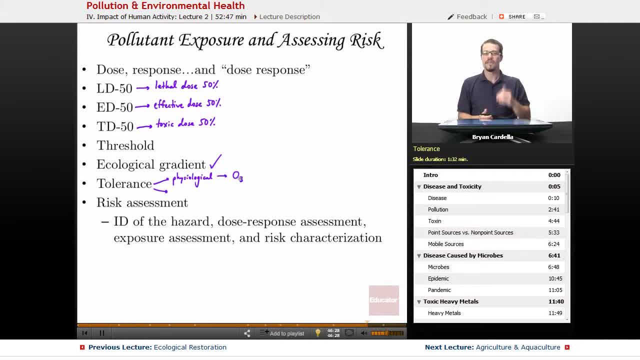 way up in the atmosphere. but there was a study done that exposed people to increasing levels of o3. they were inhaling it and at first these individuals- the vast majority of them- had respiratory distress. it was there were some negative effects but as the study went on, their bodies adjusted, their bodies. 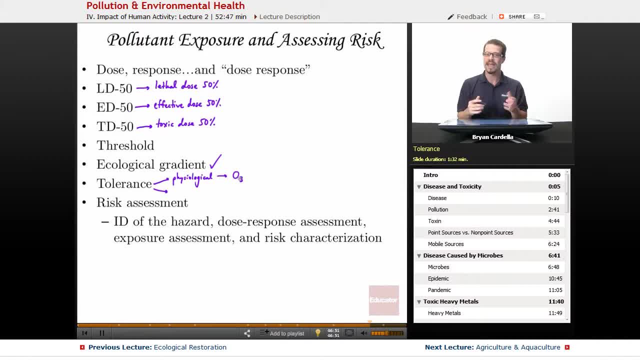 developed a physiological tolerance, where they were able to deal with it and after a while they didn't even notice that they were exposed to it. another one is genetic tolerance, and i've talked about this numerous times. uh, ddt, um, you know, ddt has been used as a pesticide in 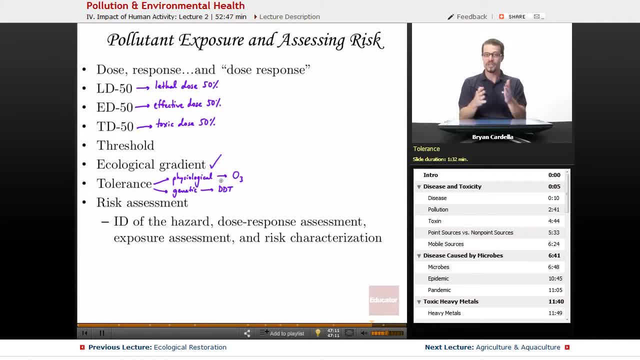 numerous cases and we've learned from our mistakes. all it takes is one individual that has a gene that allows resistance to that ddt. if they can pass on that gene to its offspring, it can spread through the entire population and then you have genetic tolerance or resistance against a. 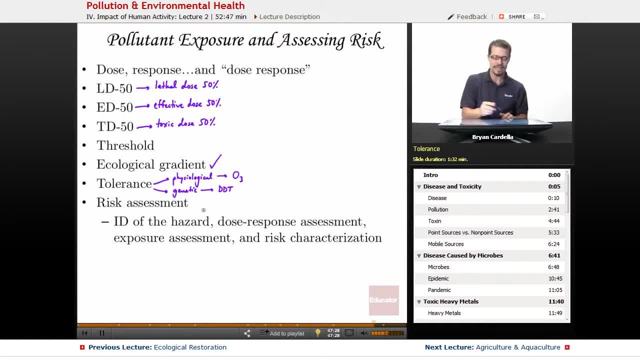 certain chemical or pollutant. all right. risk assessment anytime people are exposed to pollutants in the environment, whatever the source is, whatever the pollutant is, or the toxin identification of the hazard, meaning like hey, do we really know what's causing this negative health effect? is it the pollutant? 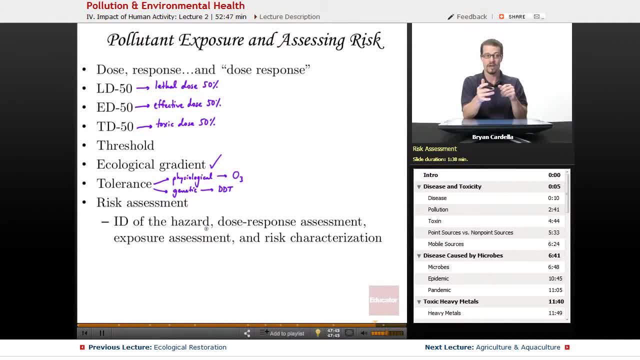 itself. uh, what do these people have in common? uh, are they all going to the same source? what is it? dose response, assessment, meaning figuring out this stuff. okay, how much of it uh is in the environment and at what level are we? are we at the point where only half of the people are getting sick? 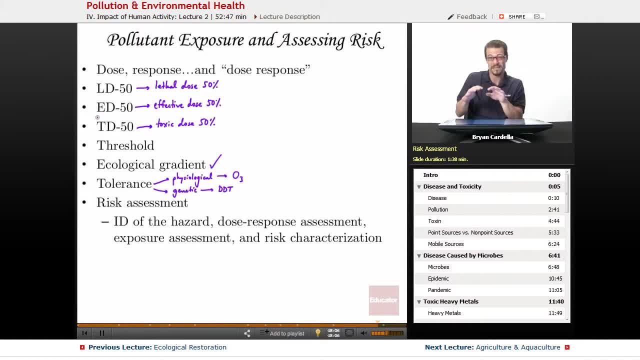 uh, is it at the toxic level? is it just at the effective level, where we're just starting to see some negative things happening in the body but we're not quite a toxicity exposure assessment? hey, how many people have been exposed? it may not just be that community um, it may be people who 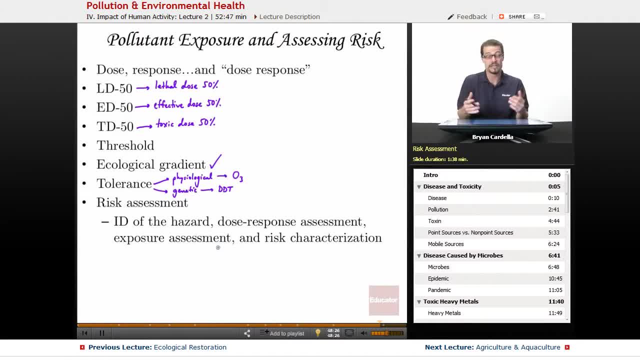 have temporarily visited there- uh, is this a tourist area? so there are a lot of things to consider with, like how many people have been exposed, and then risk characterization. when you've done these three, it leads you to making broad decisions about how to deal with this particular pollutant exposure, and it's controversial because there's 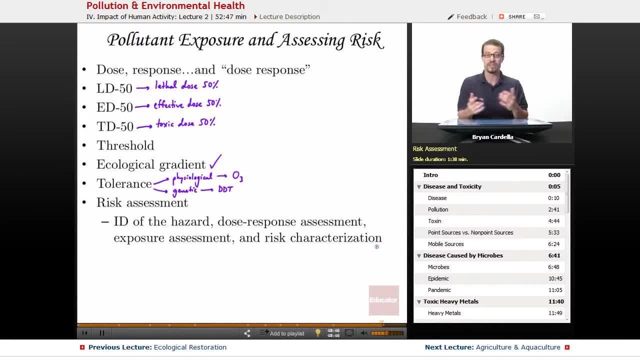 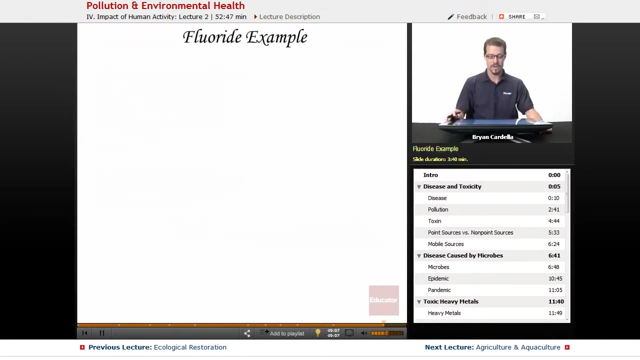 not just one way to go about doing this. different organizations have different opinions of how harmful pollutants are and what particular doses are acceptable, whether it's dioxin, like i mentioned earlier, or just vast amounts of pops and pollutants that are found in the environment. so these are very important things to consider, okay. so 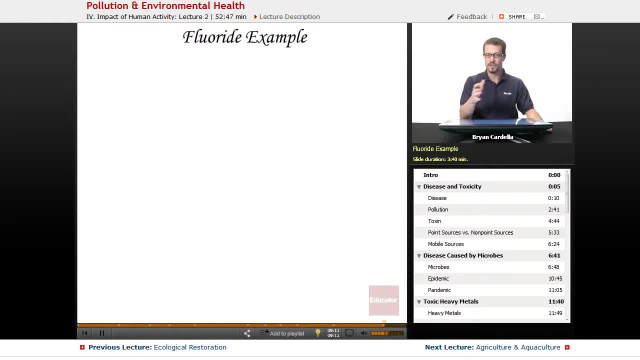 a fluoride example we were just talking about, uh, different dose response curves, ld50, ed50, td50, those things. let's look at an example now. typically, fluoride is not considered a pollutant, but depending on who you ask on this planet, you're going to get different responses. 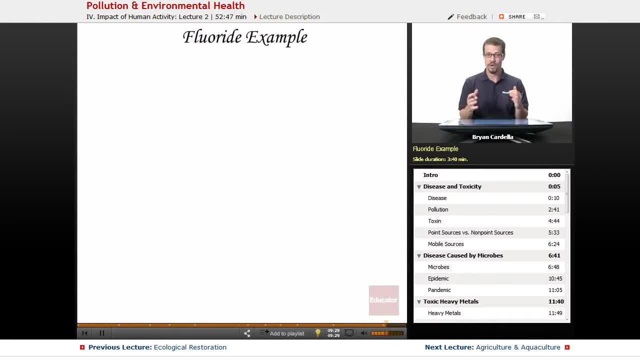 in the united states, for example, fluoride is actually in our water supply. it's in the tap water, we've grown accustomed to it. but in a lot of european countries they don't do that. they don't think it's wise. some people would argue that we have enough fluoride in toothpaste. 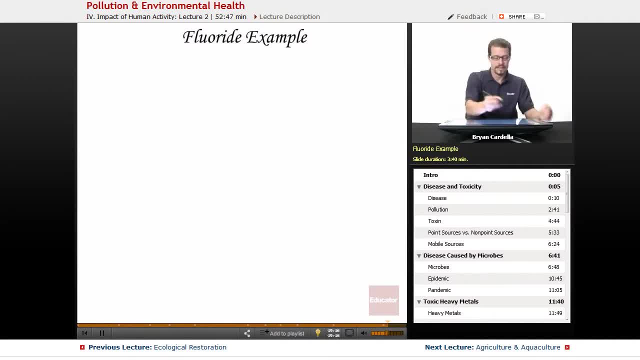 products that when we go to the dentist and get a fluoride treatment. that's enough. let me give an example of how too much fluoride could be a bad thing. okay, this is going to be kind of an atypical looking graph. here's your. your x-axis up here is going to be beneficial. 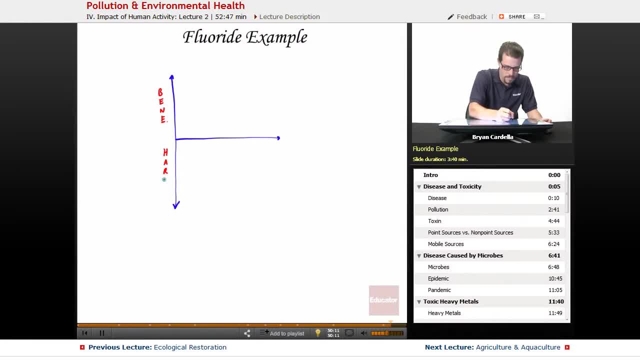 and down here is going to be harmful. okay, like a negative in a sense, and this is going to be with increased dosage. so here's dose levels. dosage: let's use black, okay. so with fluoride it could look like this, okay. so right in here is a region that we can consider optimum. that's the optimum dosage for your health, okay, because?